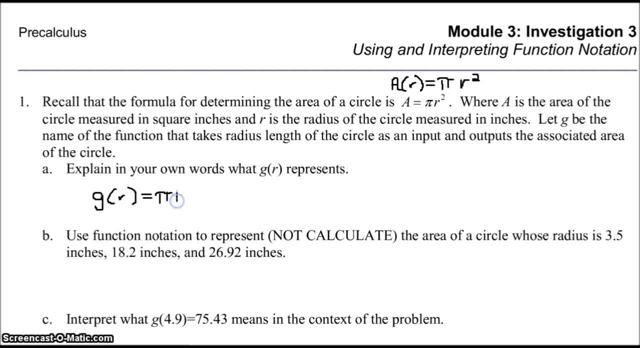 So what does g of r represent? Well, it represents the output given any particular radius input. In other words, g of r represents the set of output values for the function g. You might even say that it represents the area given a particular radius input. 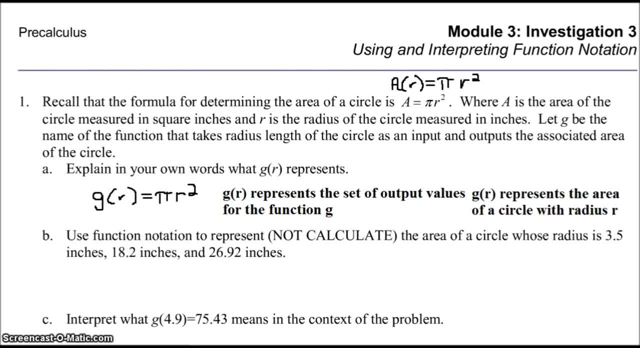 So that's our value of r. It's important that we think about input and output here. r is the input and g of r is our output. Next question says: use function notation to represent, not calculate, the area of a circle. 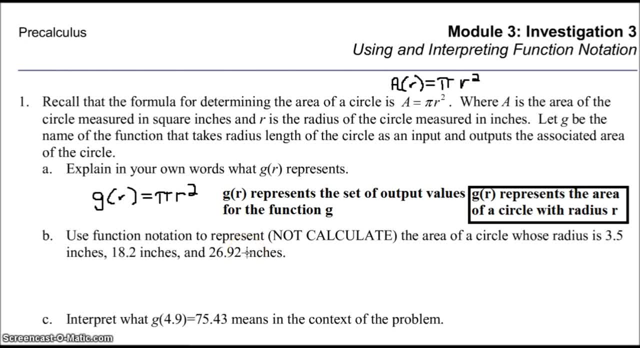 whose radius is 3.5 inches, 8.2 inches and 20.5 inches, 6.92 inches. this one's pretty simple. for the area of a circle whose radius is 3.5 inches, we represent that with G of 3.5. if our radius is 8.2 inches, we can. 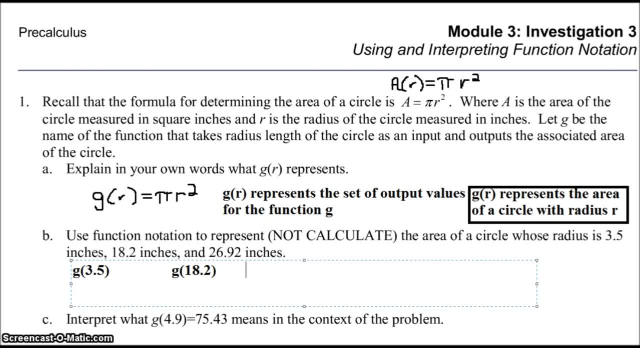 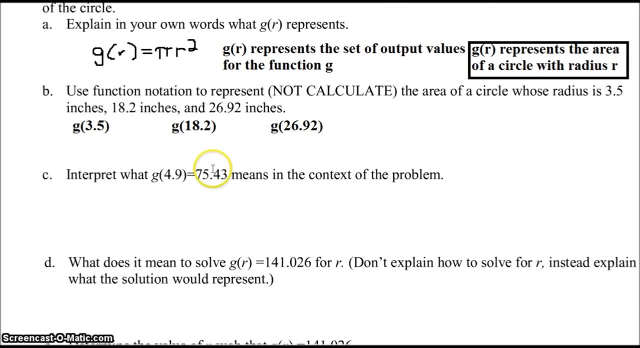 represent the area with G of 18.2. and if the radius is 26.9, 2 inches, we can represent the area with this expression here: G of 26.9, two. notice that we are picking particular values of the radius. this generic function. 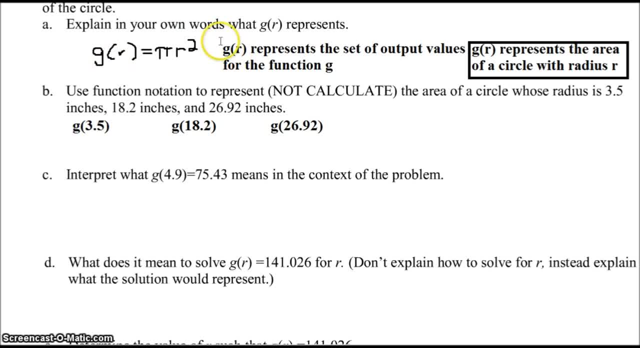 per n much works for any possible input. we can make a distinction here: G of R represents the set of output values for a function, G and that R is arbitrary. here in part B we've picked three different values of R, and those represent three different numbers, three different areas, whereas 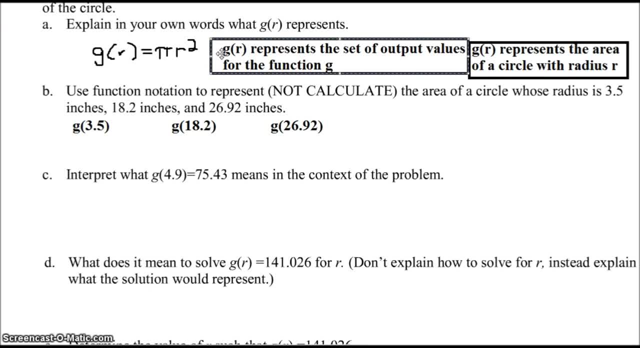 this function describes the relationship. no matter which value of R we pick, we can get the output value of the area. part C says: interpret what G of four point nine equals seventy five point four. three means in the context of the problem. so our input is four point nine. remember that that's a. 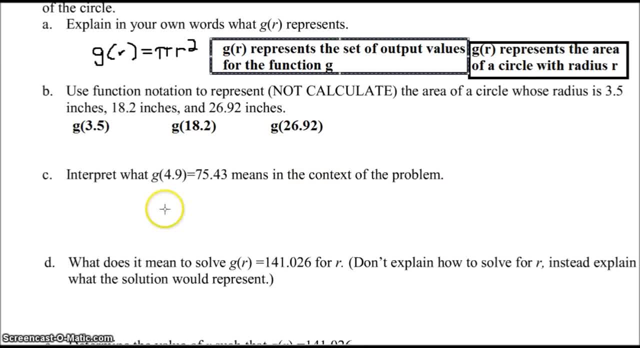 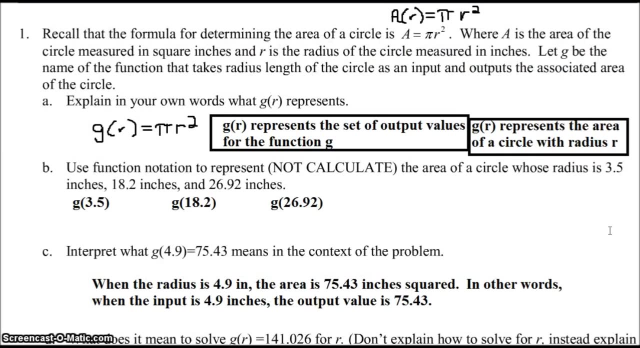 radius. so whenever we have a radius of four point nine inches, our output G of four point nine. our area is seventy five point four, three inches squared. so when the radius is four point nine inches, the area is seventy five point four, three inches squared. you could also say that when the input is four point nine inches, the output 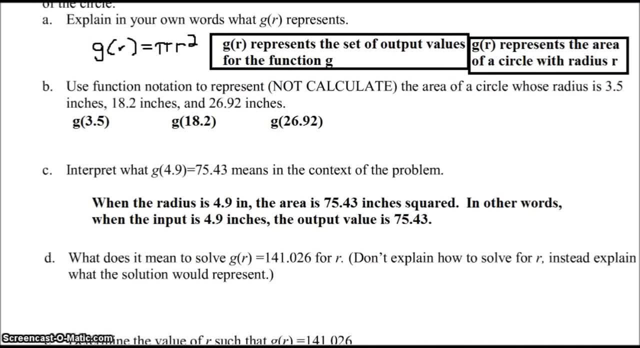 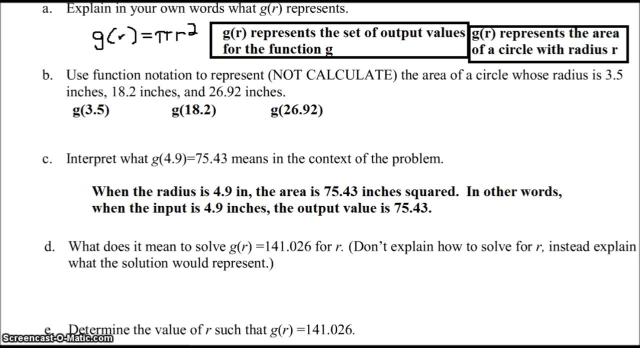 value is seventy five point four three. what does it mean to solve? G of R equals 141.026 for R. don't explain how to solve for R. instead explain what the solution would represent. so this of R, remember that represents the area of a circle with radius R and if the area is 141.026, 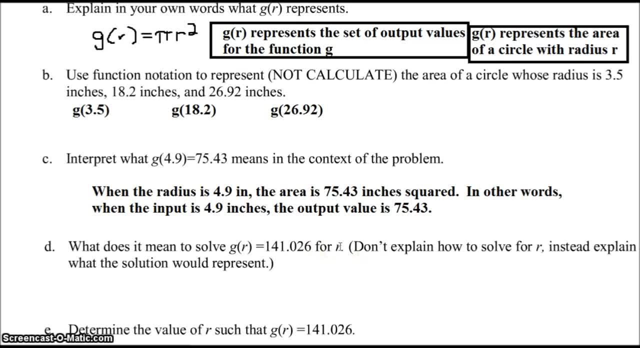 for this particular value of our. if we solved for are, that would tell us the radius, we would need to have an area of 141.026 eyes for our circle. so if we find the value of R says that G of R equals a hundred and forty one point zero two. 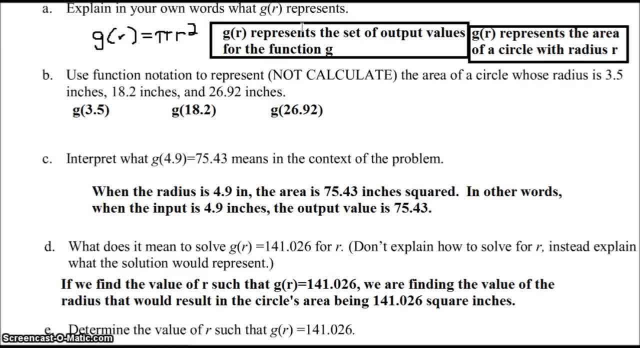 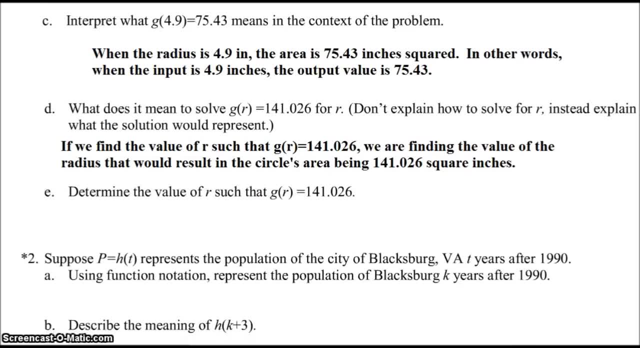 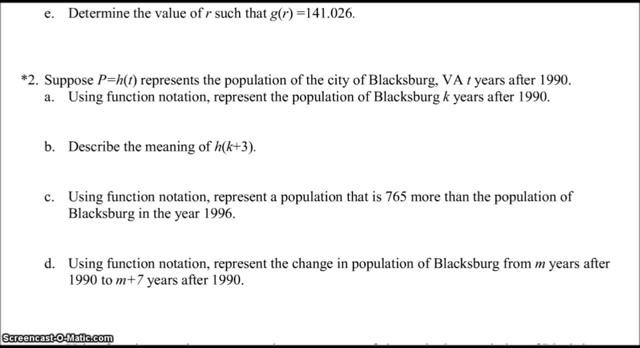 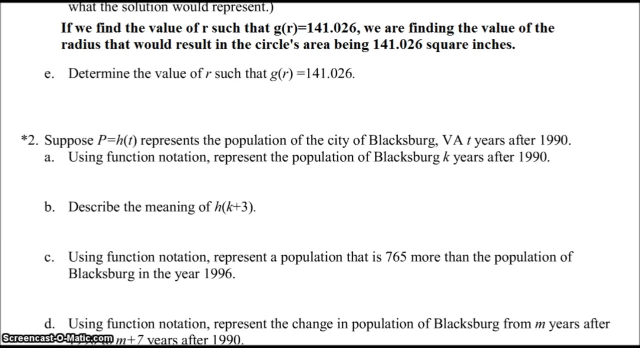 What we are finding is the value of the radius. that would result in the circle's area being 141.026 square inches Determine the value of r, such that g of r equals 141.026.. So what we're going to do now is figure out what that radius would be. 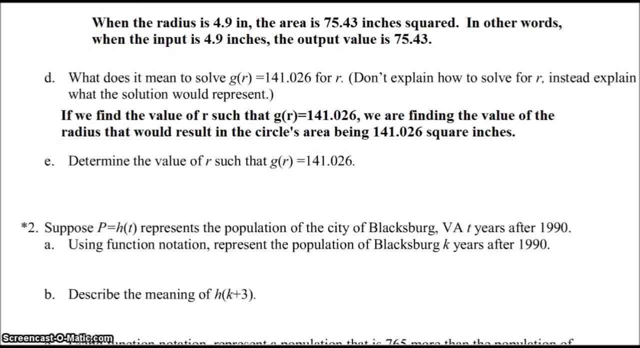 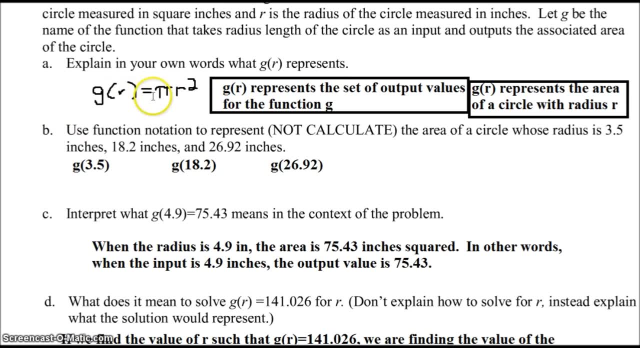 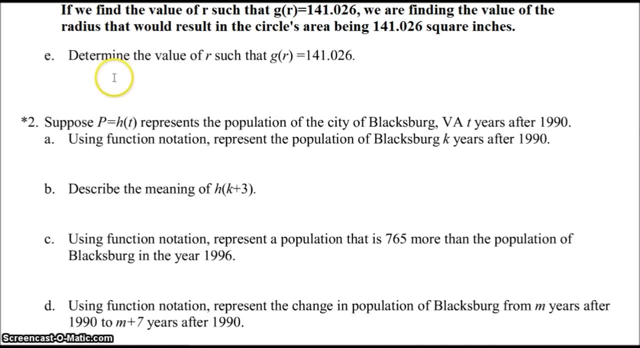 So we simply think about what our function, g of r is. Remember that g of r is the area of the circle. It's equal to pi r squared right here. So g of r equals pi r squared and we know that g of r is 141.026.. 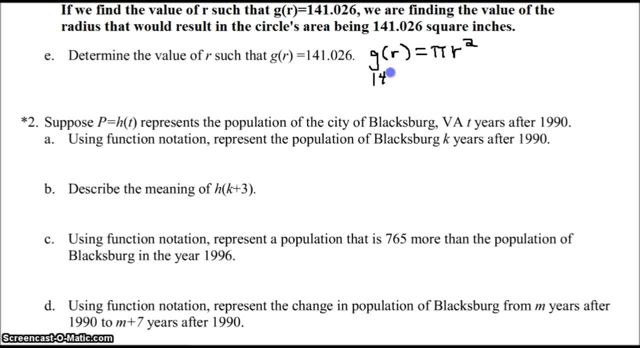 So we know that our output value g of r is 141.026.. And that's equal to pi r squared. Next, we need to solve this equation for r. So I'm going to give us a little bit of room. I moved what we've done so far to the right and started again here on the left. 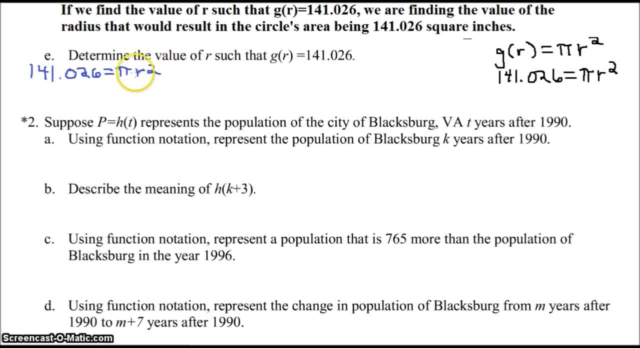 If we want to solve for r- notice r is being squared- then it's being multiplied by pi. We need to undo this equation First. we can divide both of our sides by pi. So we have 141.026 divided by pi is equal to r squared. 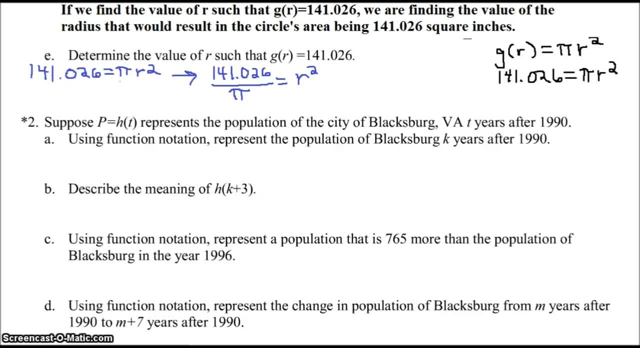 So to find the value of the radius we just need to take the square root of both sides. Since we have the radius is squared, We can undo that square with the square root. We can just think: well, if r squared equals this number, then r equals the square root. 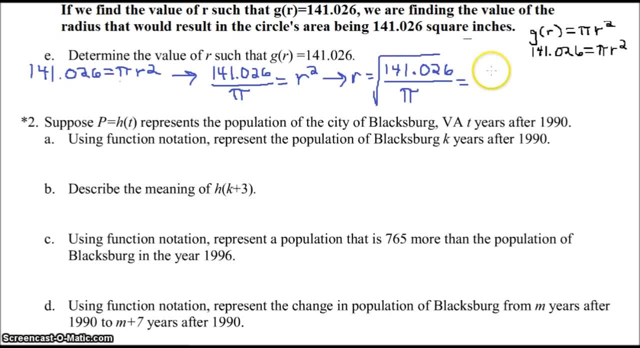 of this number. So r is the square root of 141 over pi, And note that we don't need a plus or minus here, because the radius can only be positive. Then if you use your calculator, that's about 6.70 inches. 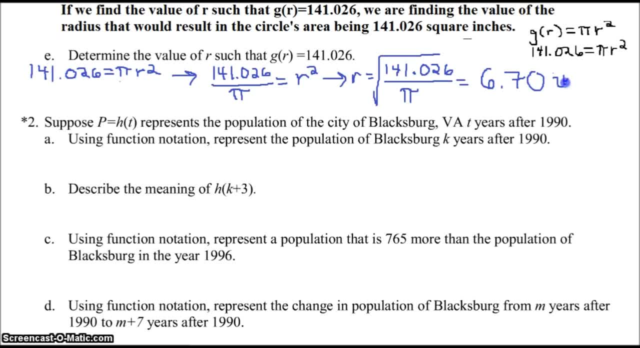 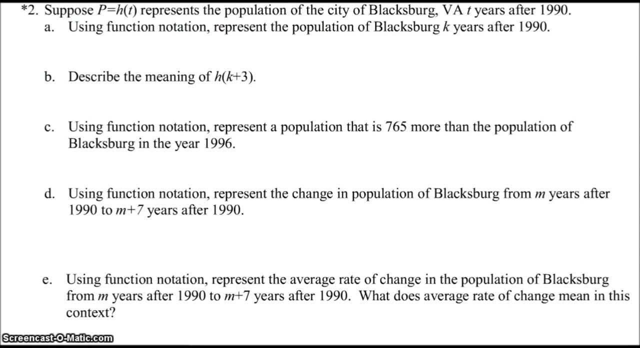 Okay, 6.70 inches. So that's the value of the radius. that will give us an area of 141.026 square inches. Question 2. Suppose p equals h of t represents the population of the city of Blacksburg, Virginia, t years. 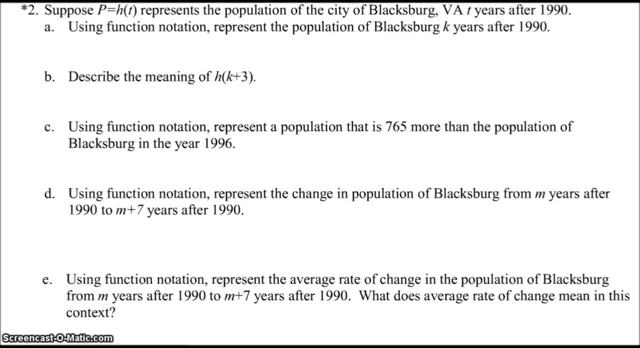 after 1990.. Using the function notation, represent the population of Blacksburg k years after 1990.. Take a second to think about this. The key is just understanding the problem If we want to represent the population of Blacksburg k years after 1990.. 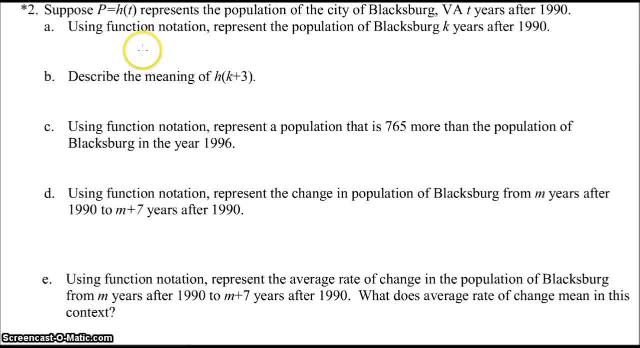 Well, our function h represents the population of the city of Blacksburg, Virginia t years after 1990.. Okay, So if we want to find out what's the population in year k, We just plug k into the function. That's it. 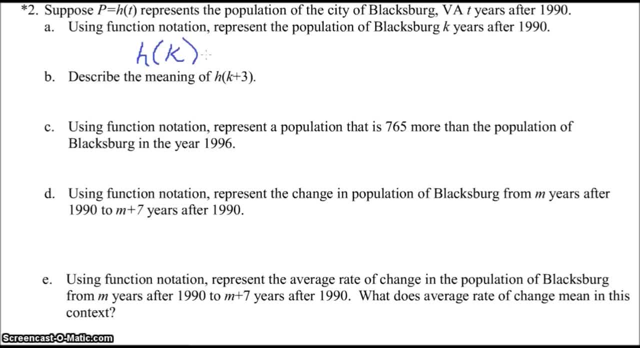 Part b Describe the meaning of h of k plus 3.. So k plus 3 is our input. Recall that that's the number of years after 1990.. So let's see k plus 3 just means k plus 3 years after 1990.. 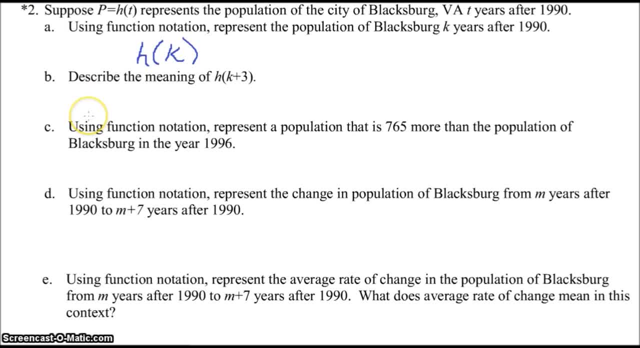 And remember that our function h represents the population of the city of Blacksburg, So h of k plus 3 represents the population of the city of Blacksburg, k plus 3 years after 1990.. Okay, So Part c, Part c. 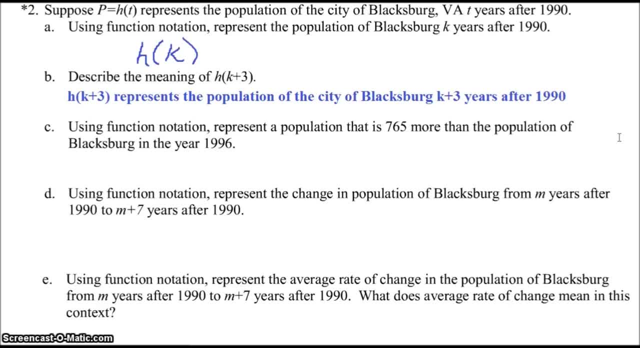 Using function notation, represent a population that is 765 more than the population of Blacksburg in the year 1996.. There's a couple things going on in this sentence. First, 765 more than the population of Blacksburg in the year 1996 tells us that we just need. 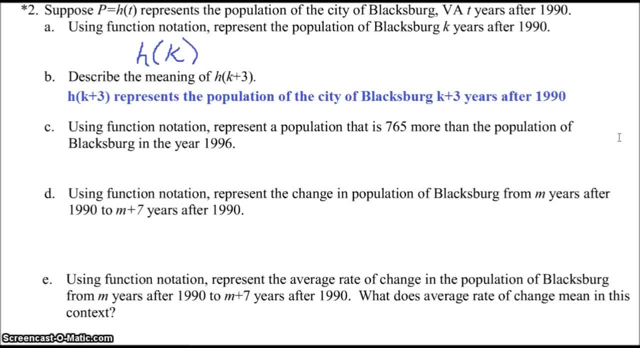 to add 765 onto the population of Blacksburg in the year 1996.. So how do we find that, or how do we represent the population of Blacksburg in the year 1996? Well, remember our function h. it tells us the population t years after 1990.. 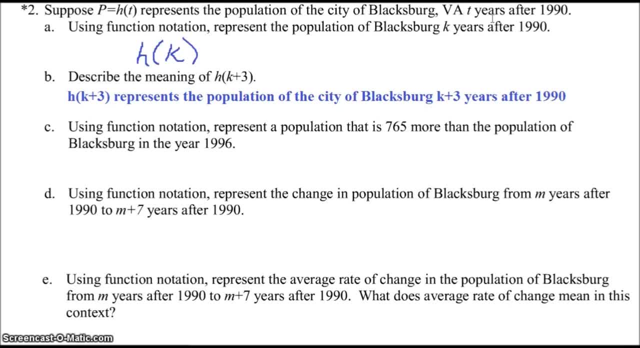 So in 1996, that would be 6 years after 1990.. So we need t equal to 6.. Okay, So we can simply write h of 6. That will tell us the population of Blacksburg in the year 1996.. 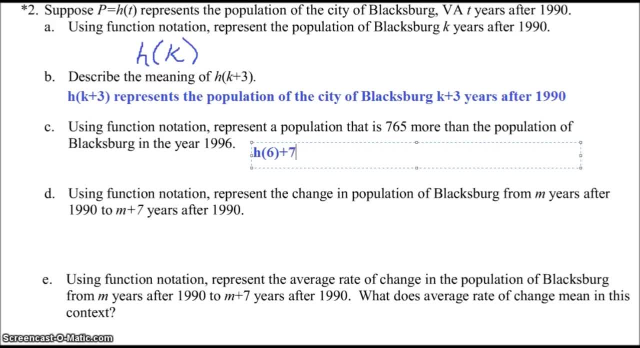 But we want to represent a population that is 765 more than that population Simply h of 6 plus 765.. Part d, Using function notation, represent the change in population of Blacksburg from m years after 1990 to m plus 7 years after 1990.. 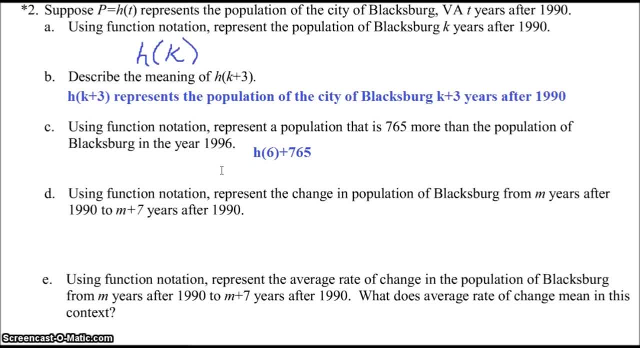 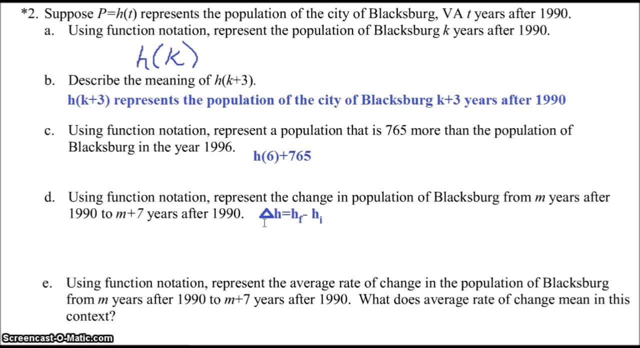 So here we're interested in a change in population. Recall that a change is the final value minus the initial value. So remember our delta h is what we use to represent change. So delta h equals h final minus h initial. So the final population that's going to be m plus 7 years after 1990.. 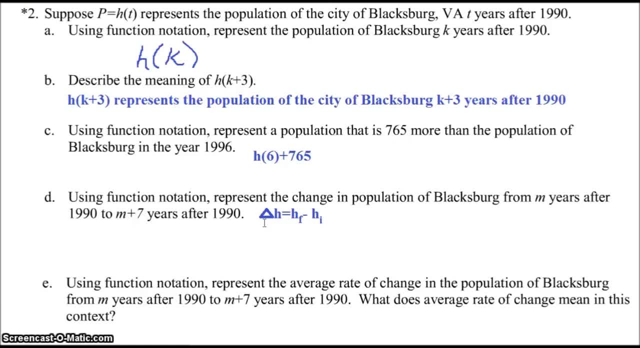 We can represent that simply with h of m plus 7.. And then m years after 1990, that's just h of m. So there's our population, Okay, Okay, Okay, Okay. So that's our final population minus our initial population: h of m plus 7 minus h of m. 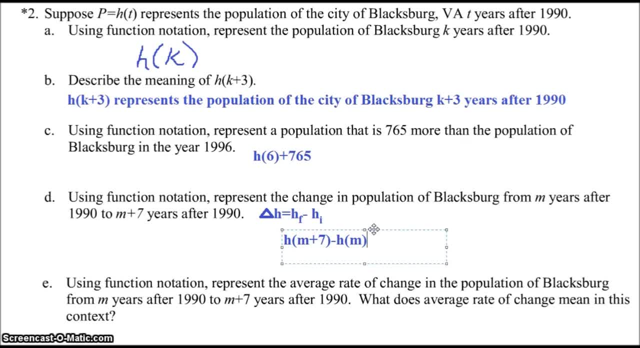 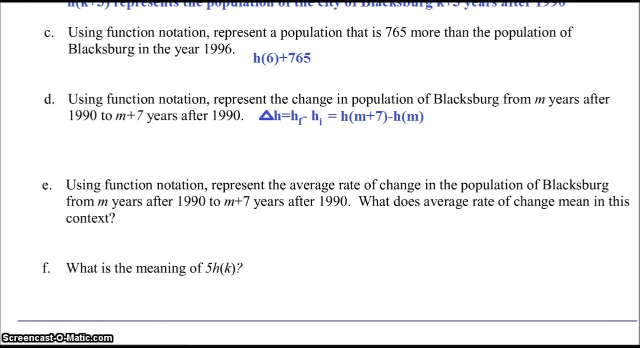 That represents the change in population of Blacksburg m years after 1990 to m plus 7 years after 1990.. We can even put an equal sign here. Next, or part e, we need to represent the average rate of change in the population of Blacksburg. 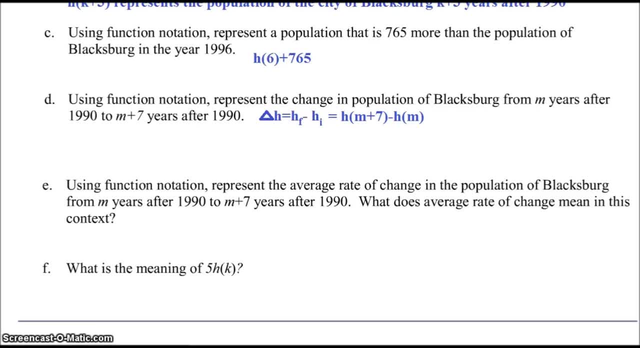 from m years after 1990 to m plus 7 years after 1990, just like in the previous problem. But now we want the average rate of change, And remember that the average rate of change is the constant rate of change needed to. 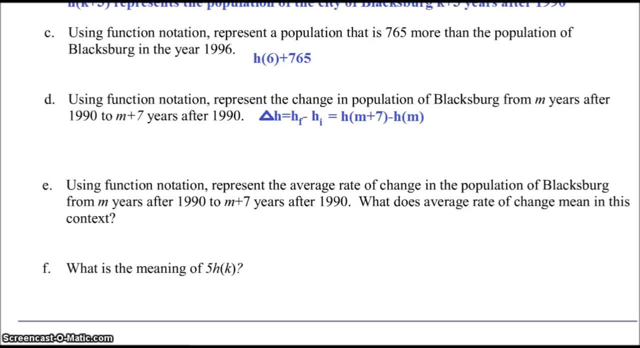 in this context, have the same change in population in the same amount of time. So to find the average rate of change we simply calculate the ratio, a rate of the change in height over, not the change in height, I'm sorry- the change in population over the. 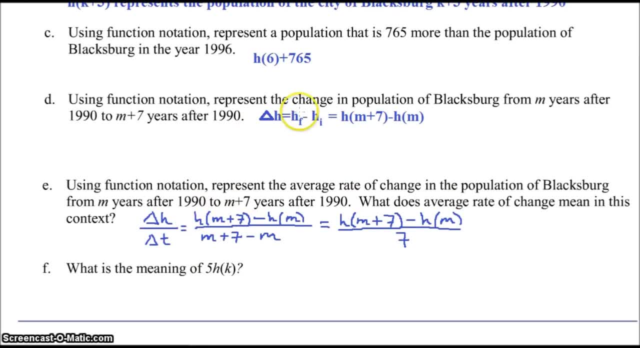 change in time, And that change in population, as we saw from the previous problem, is just h of m plus 7 minus h of m divided by the change in time. well, the final time was m plus 7 and the initial time was m. 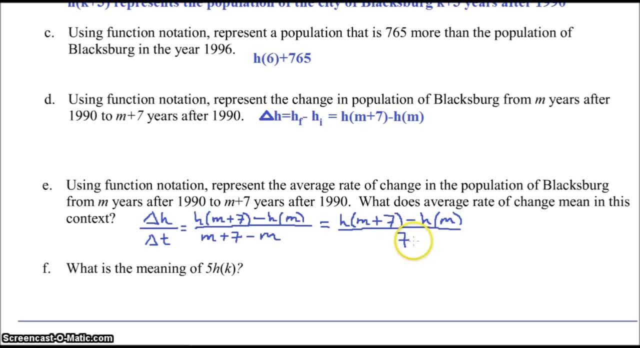 Notice that when we subtract those the m's cancel out, we get 7, and that 7 just represents the change in time, And that change in time from year m to m plus 7, there was just 7 years in between. 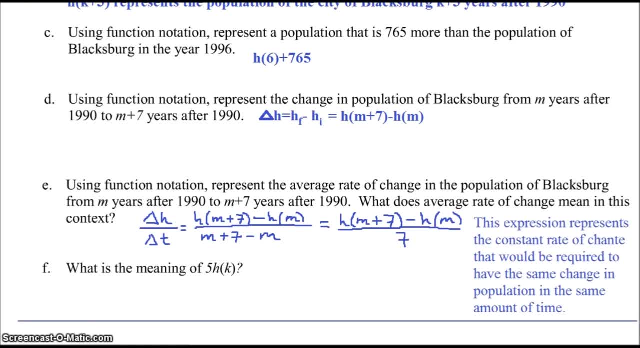 And this is our average rate of change. This expression represents the constant rate of change that would be required to have the same change in population in the same amount of time, And this needs to be a g. Oh well, The population may not be changing at a constant rate. 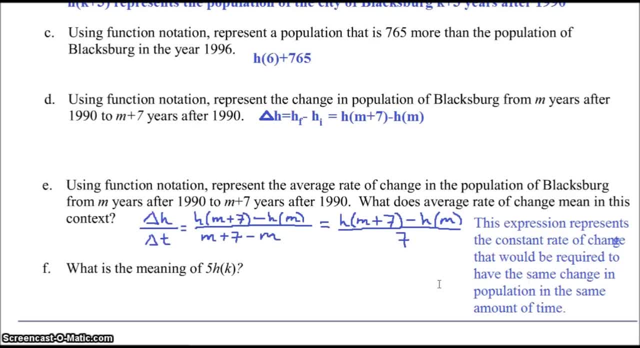 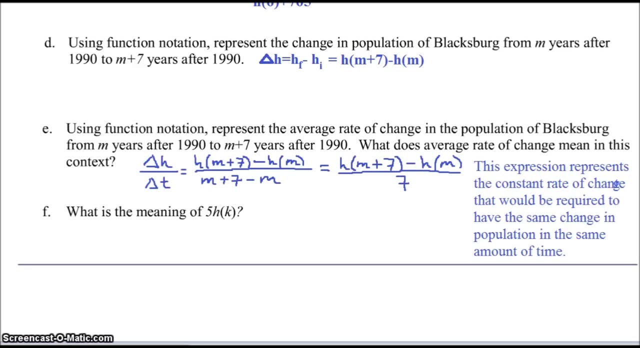 But what this expression tells us is the constant rate of change, that we would need to have the same change in population in the same amount of time. Part f: what is the meaning of 5 h of k? That's just 5 multiplied by h of k, and remember the input is just k years after 1990.. 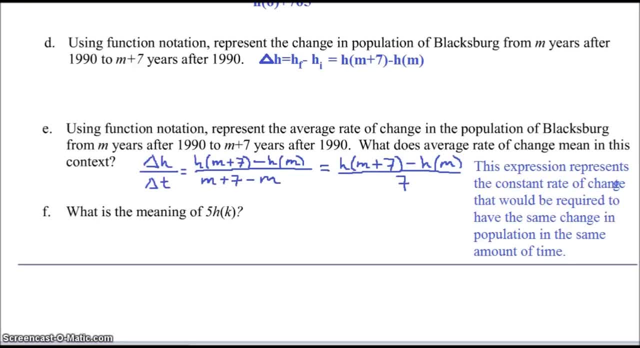 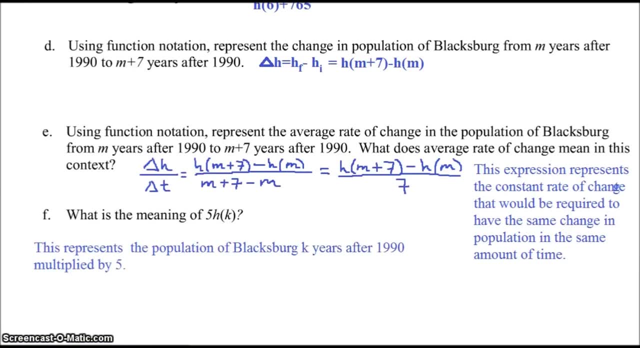 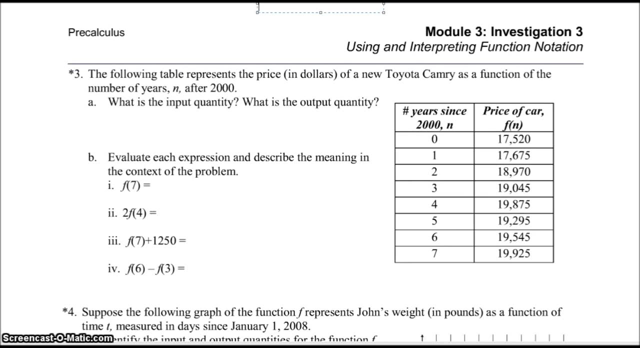 So we're essentially taking the population k years after 1990, and multiplying it by 5.. Number 3.. The following table represents the price in dollars of a new Toyota Camry as a function of the number of years in after 2000.. 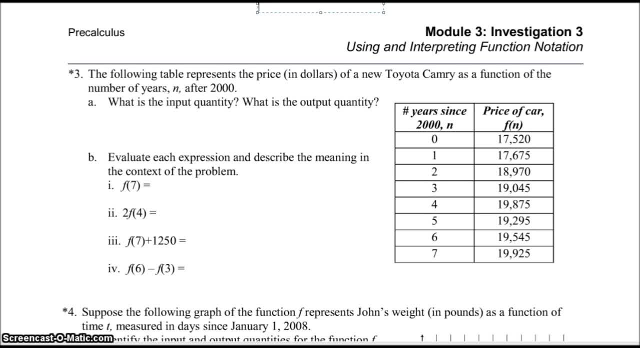 What is the input quantity and what is the output quantity? So recall our definition of function. When we say a new Toyota Camry as a function of the number of years in, then Toyota Camry is the dependent variable. the number of years in is the independent variable, the price. 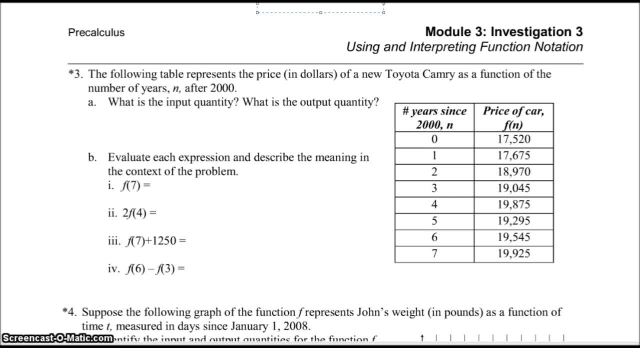 of the Toyota Camry is the output and the number of years in is the input. Part B says to evaluate each expression and describe the meaning in the context of the problem F of 7.. F of 7 represents the output of our function when the input is 7.. 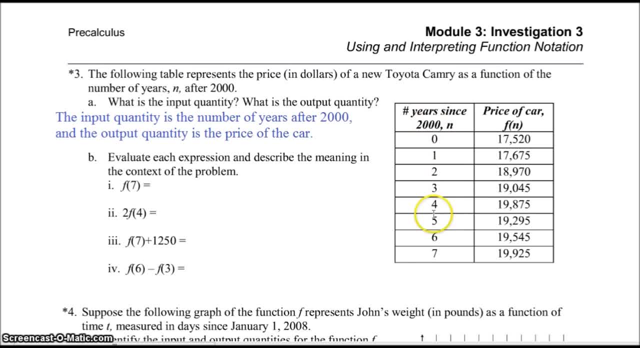 Now we know that the input is the number of years since 2000,. so our input is 7, and when we have that, So our particular input, our output is $19,925, the price of the car and 2007 is $19,925. 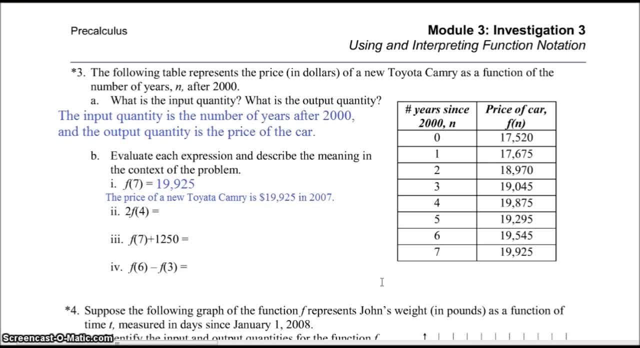 Now part 2 is 2 times F of 4.. First of all, F of 4 represents the price of the car. Four years after 2000,. or in 2004,, we can look at our table and see the price of the. 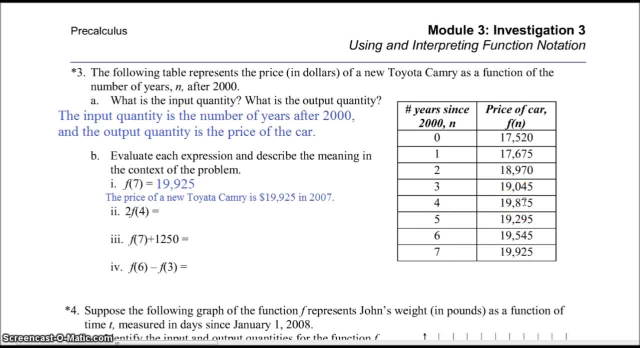 car is $19,875.. That 2 times F of 4 just means that it's twice the price of the car in 2004.. Maybe we're buying two cars or something. So we could say the cost of two Toyota Camrys in 2004 is $39,750. 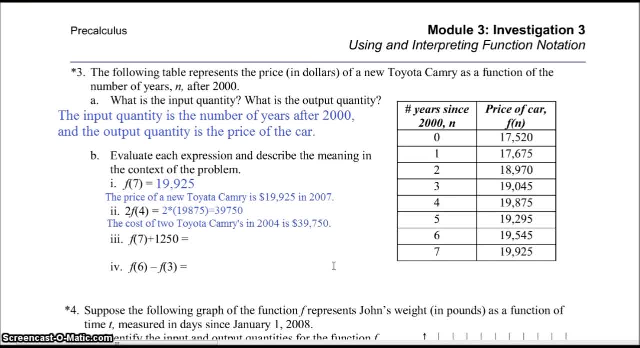 Part 3, F of 7 plus $1,250.. Well, F of 7 is just the price of the car seven years after 2000.. That's $19,925 plus $1,250. And that comes out to $21,175. So we can say that the cost of a new Camry in 2004.. In 2007, plus an additional $1,250, is $21,175.. In a real-world situation this could be the price of the car plus perhaps interest on. 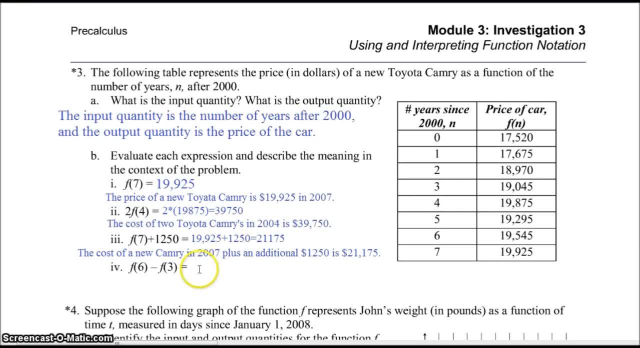 a loan In part 4, we have F of 6 minus F of 3.. So the price of a Camry in 2006,, which is $19,545, minus the cost of a Camry in 2004,. 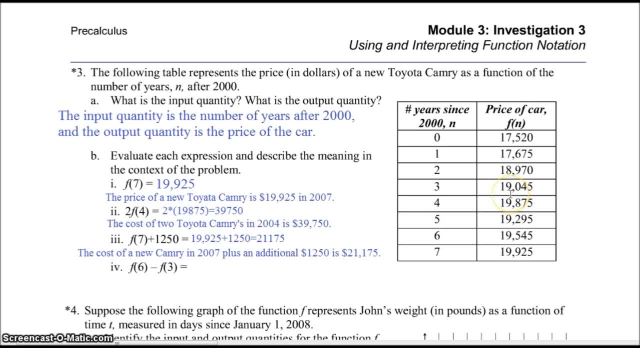 is $19,545. So that's $19,545. So that's $19,545.. In 2003,, $19,045. So that comes out to $500. And we could say something like the cost of a Camry increased in $500 from 2003 to 2006.. 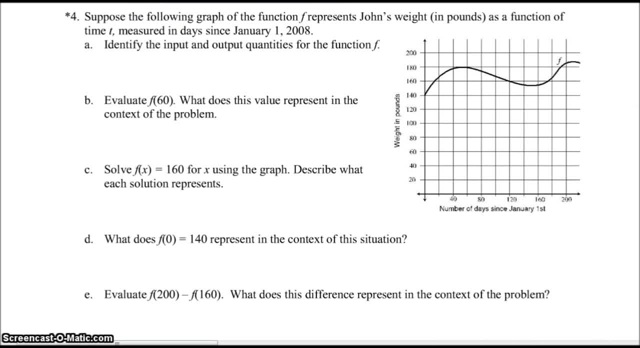 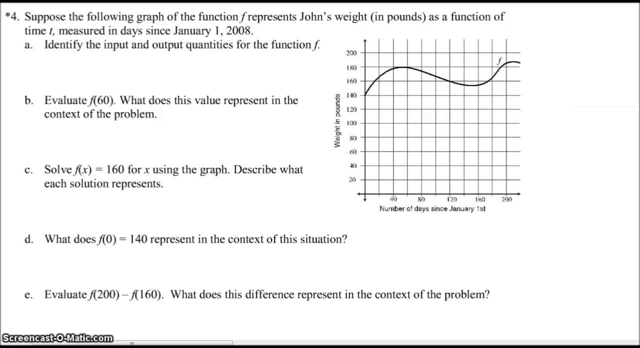 Number 4.. Suppose the following graph of the function: F represents two cars: F of 7 plus $1,250.. F of 6 minus $1,250. And we have F of 7,250. So the cost of the car is $20,200.. 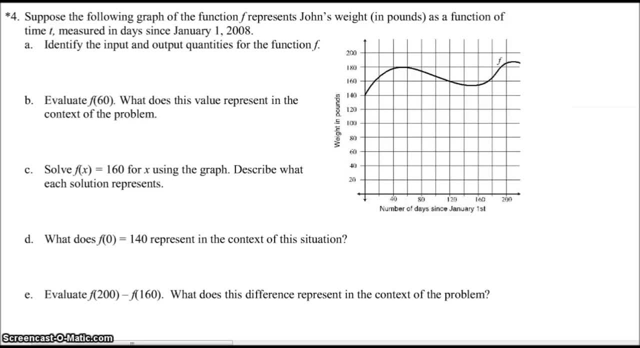 Remember that F of 7,250 is $32,200.. So T of 7,250 is $한다, which, if there are other numbers- of 5,250.. So the cost of the car is $40,000.. So we know that F of 7,250 comes from the $30,000 left over. 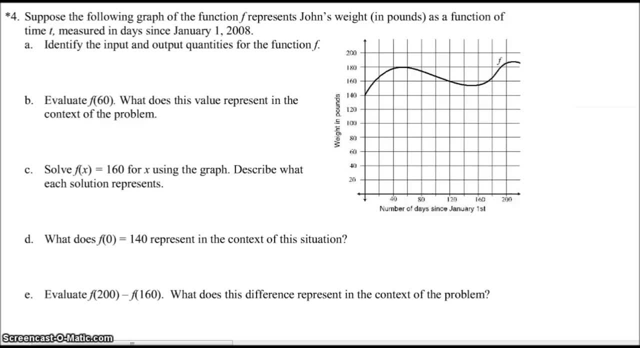 So the cost of the car is $10,000.. So we know that F of 5,250 is $10,000.. Notice that the value of F of 6,250 is $10,000.. So T of 6,250 is $10,000. 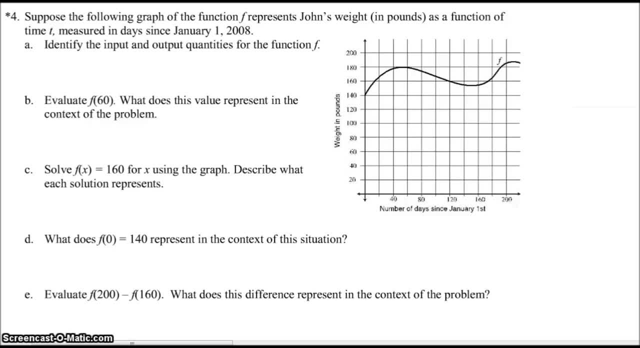 So all of these numbers above the cost of the car is F of 6,250.. So that's the cost of the car. The cost of the car is $20,000.. notice that we have john's weight as a function of time t. so the time t is the input and john's 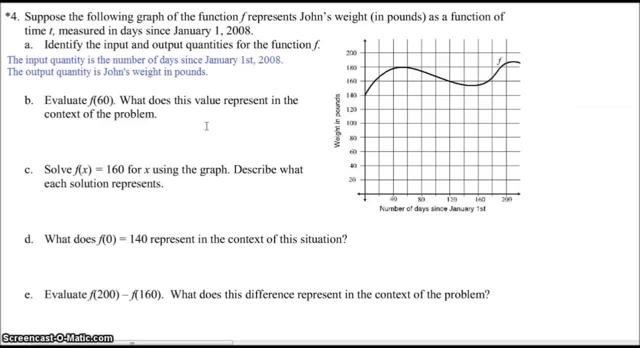 weight is the output. part b: evaluate f of 60.. what does this value represent in the context of the problem? so simply take a look here. here's um. when the input is 60, that's 60 days since january 1st- we can go up to our function and take a look at the corresponding y value, which is about: 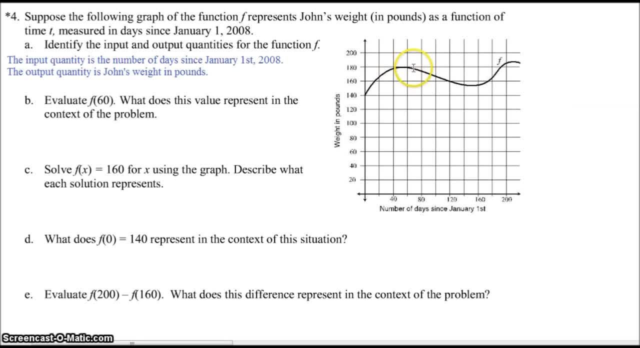 oh, almost 180. um, we could say 179 or something. so f of 60 equals 179 and this means that john weighs 179 pounds 60 days after january 1st. so solve: f of x equals 160 for x using the graph, describe what each solution represents. so if we 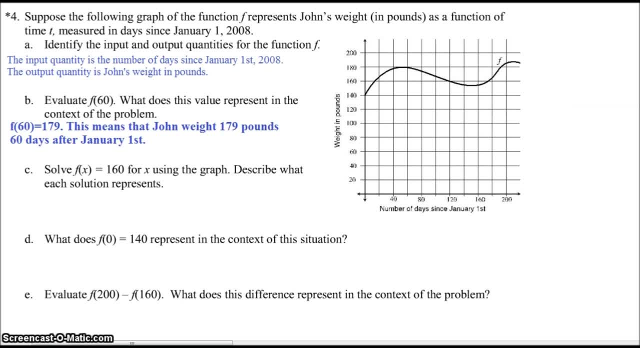 look at our graph um. when f of x, the function output is 160.. that means that john's weight in pounds is 160.. we can see that that occurs here and it also occurs right here, and right here there's three corresponding x values. that means there's three different days. 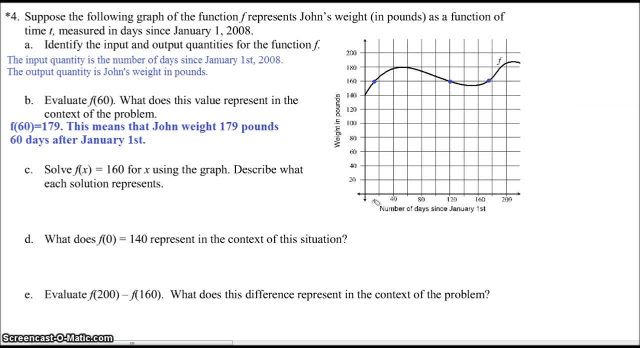 when john's weight was 160.. we see that those are, let's see about um a little less than 20, maybe like 17.. i'm right at 120, and let's see a little less than 180, maybe 178.. so again, x is 17,, x is 120,, x is 178,. this means that 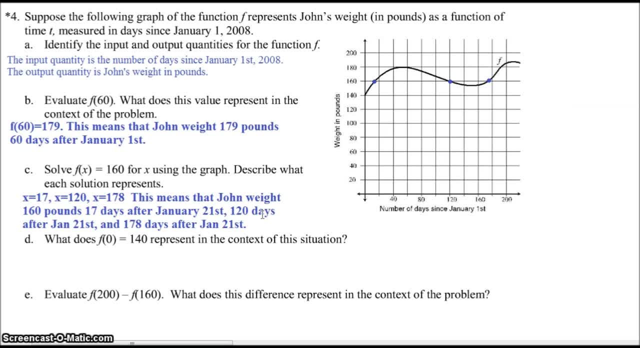 john's weight. um, um, sorry, I keep spilling weight or weighed for some reason. john weighed 160 pounds 17 days after January 21st. he also weighed 160 pounds 120 days after January 21st and again 178 days after january 21st. 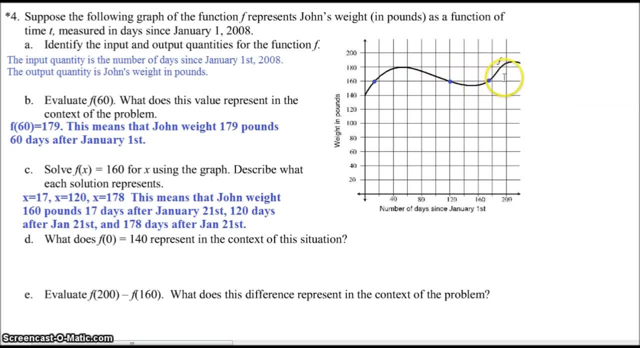 we can see that his weight is changing as the days go by. Part D: what does F of 0 equals 140 represent in the context of this situation? so F of 0 is 140. that simply means that zero days since January 1st or on January 1st, John weighed. 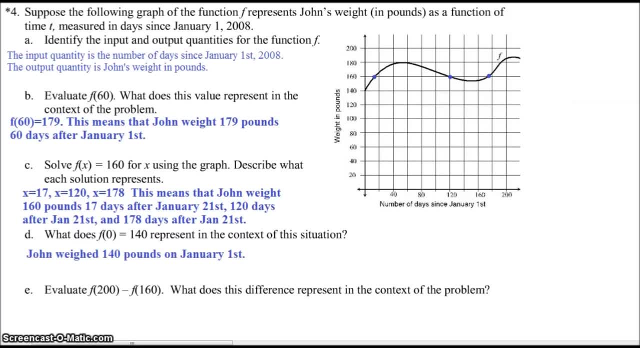 140 pounds. in part. E were asked to evaluate F of 200 minus F of 160. think about what this difference represents in the context of the problem. first we need to calculate F of 200 and looking at our graph here, when the input is 200, 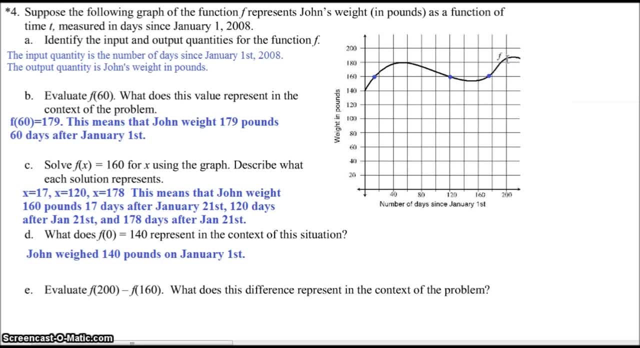 the output is maybe about 185. then we need to calculate F of 160. when the input is 160, the output just below 160, maybe about 155. so next we can calculate the difference: F of 200 minus F of 160 equals 185. 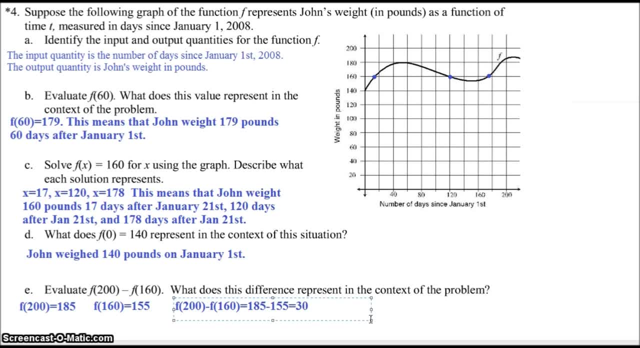 minus 155 or 30. so what does that mean? so what does that mean? what does this difference represent in the context of the problem? well, we know that it's a difference in weight and if we look at our graph, from 160 day 160 to day 200, 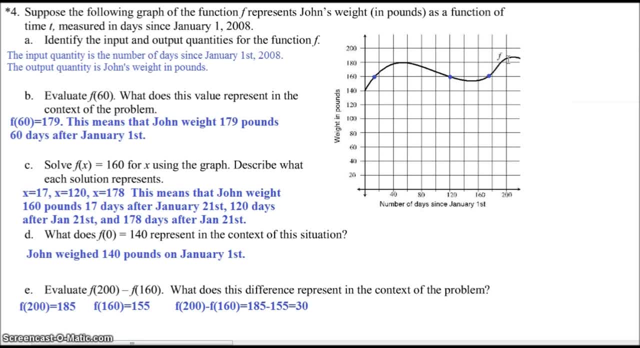 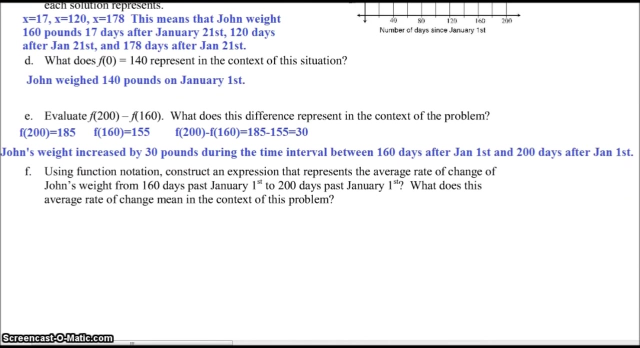 we can see that his weight increases. so we know that John's weight increased by 30 pounds from, let's see, 160 days after January 1st to 200 days after January 1st. so over the course of those 40 days his weight increased by 30 pounds. 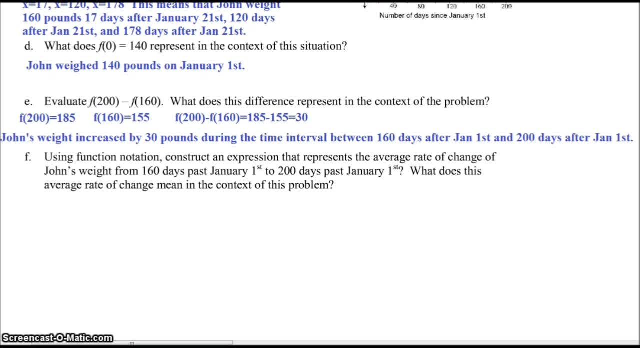 now using function notation to construct an expression that represents the average rate of change of John's weight from 160 days past January 1st to 200 days past January 1st. what does this average rate of change mean in the context of the problem? 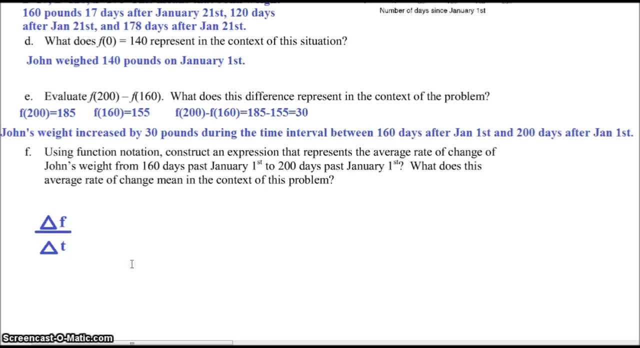 now, when we want to find average rates of change, we're just looking at the rate at which the function output value corresponds to the rate at which the function input value changes. delta F over delta T, the change in the function value divided by the change in time. 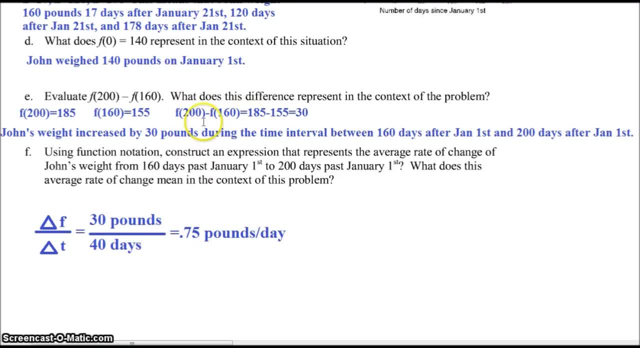 So from the previous problem we found that F of 200 minus F of 160 was 30. The change in the weight was 30 pounds and then the change in time we can find just 200 minus 160 is 40 days. 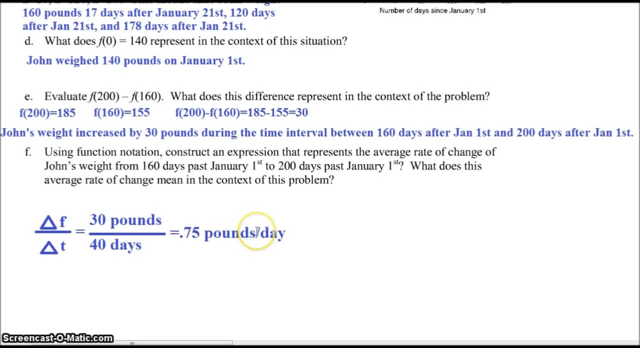 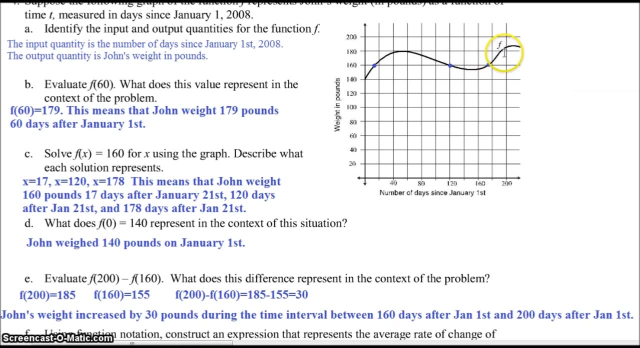 So 30 pounds over 40 days is 0.75 pounds a day. So how do we interpret what this means in the context of the problem? Well, notice that John's weight fluctuated over those 40 days. He didn't have a constant rate of change, because there's not a linear function here. 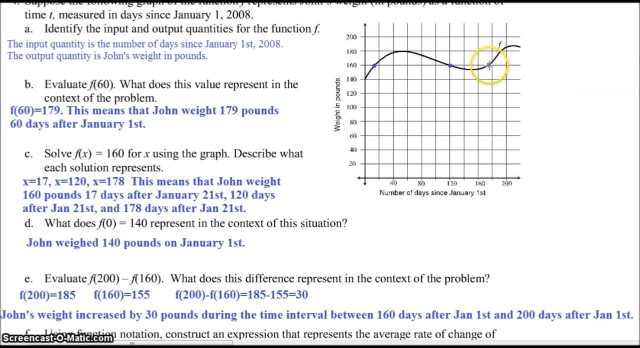 But if we want to consider the constant rate of change that John's weight fluctuated over those 40 days it would be needed such that he could gain the same amount of weight in the same amount of time, equivalent to the slope of the line connecting those two points. 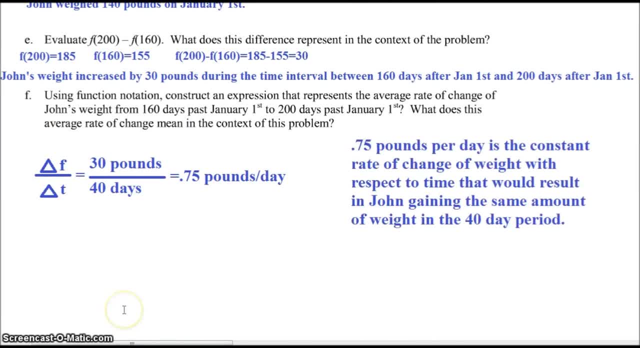 That's what we have here with the 0.75 pounds. So 0.75 pounds per day is the constant rate of change of weight with respect to time. that would result in John gaining that same amount of weight, or 30 pounds, in the 40-day period. 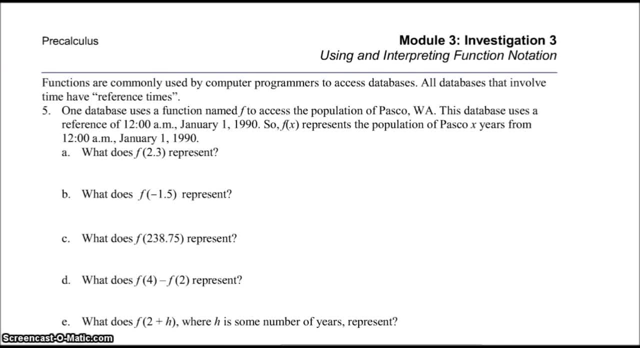 Number five says that functions are commonly used by computer programmers to access databases. All databases that involve time have reference times. One database uses a function named f to access the population of Pasco Washington. This database uses a reference of 12 am January 1, 1990.. 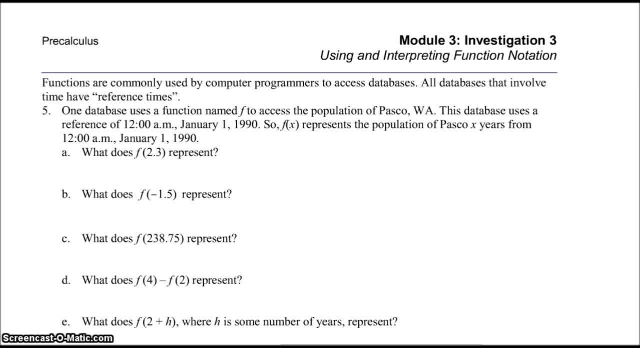 So f of x represents the population of Pasco x years from 12 am January 1, 1990.. So what does f of 2.3 represent? Well, that's simply the population of Pasco 2.3 years from 12 am January 1, 1990.. 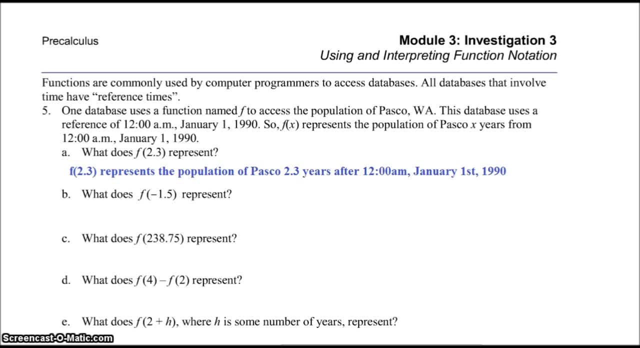 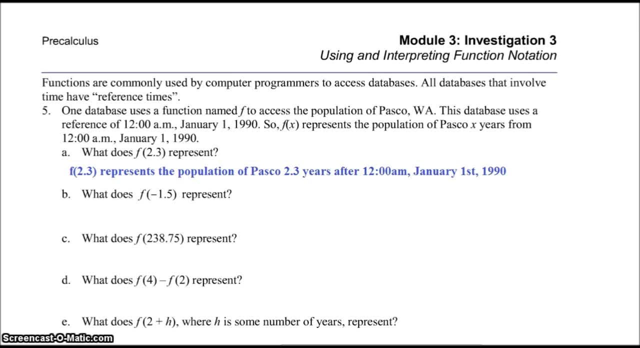 five years from 12 am January 1st 1990. so the negative here with the time just means it's 1.5 years before 12 am January 1st 1990. Part C: what does F of 238.75 represent? 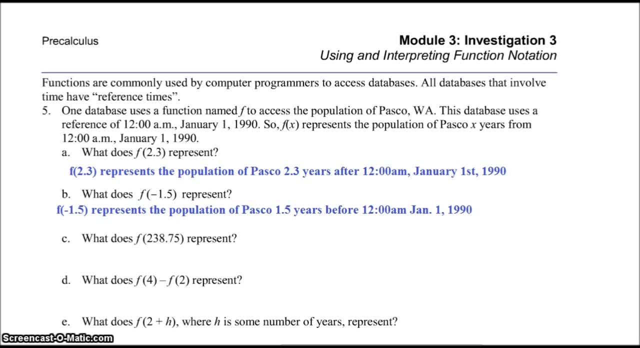 That's simply the population of Pasco, 238.75 years after 12 am January 1st 1990. What does F of 4 minus F of 2 represent? This simply represents the change in population from two years since 1990 to four years. 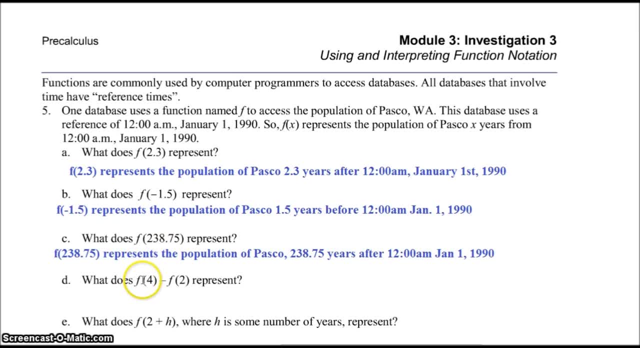 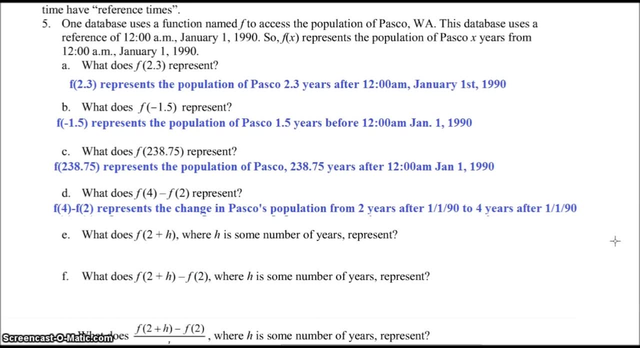 since 1990.. We could think about it as a final population value minus an initial population value or the change. We can also think about this in terms of the actual number of years. Two years after 1990 will be 1992 and four. 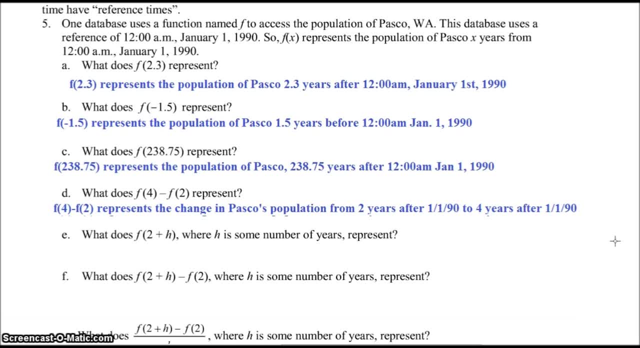 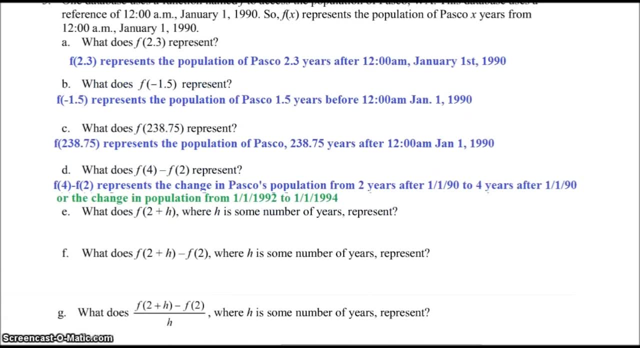 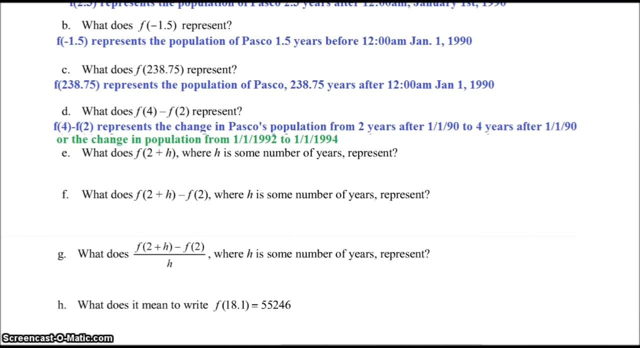 years after will be 1994.. Okay, so parts E, F and G kind of interesting. What does F of 2 plus H or H plus two years, in particular a sample, the H of some number of years, represent? Well, it's obviously. 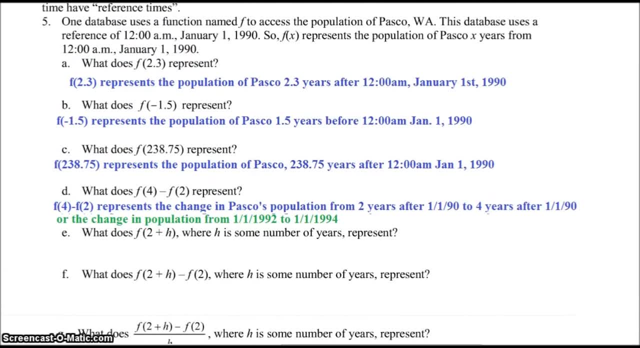 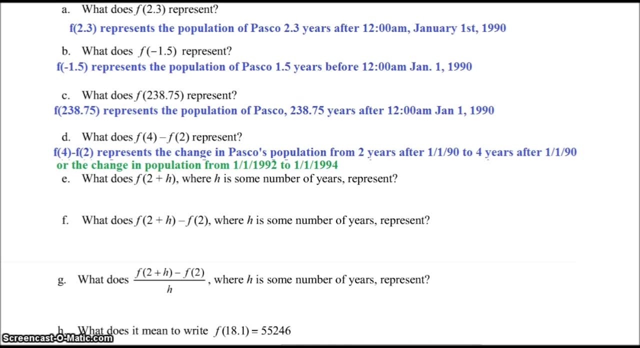 h plus two years, the population age plus two years since 1990. but we might want to try to put this in a little bit more context, So also notice that we need to. let's see like f of 2 would be two years after 1990 or. 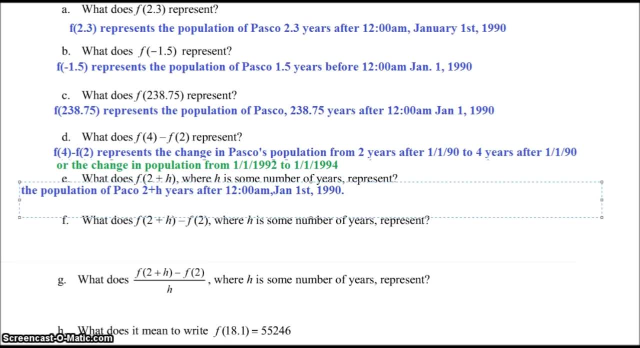 1992.. and then we're adding eight years onto that year, so we could say something like the population of paco eight years after 12 am january 1st 1992. so that's, that's alpha a. but they're actually not just alpha, that's also animal. 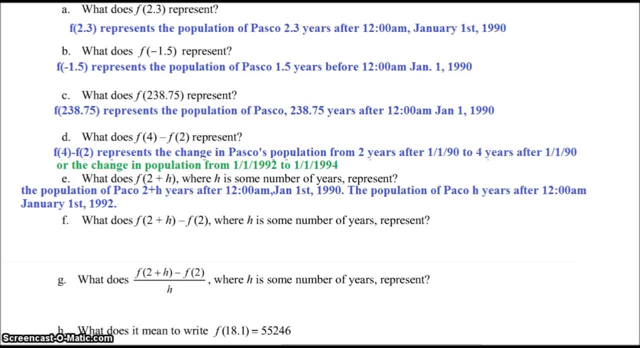 so for part f, what does f of two plus h minus f of two, where h is some number of years, represent? well, that's simply going to be the change in population from two years after 1990 to 2 plus 8 years after 1990. 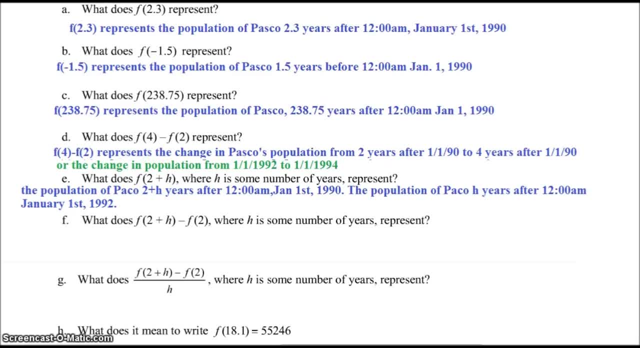 the change in population from January 1, 1992 to sometimes 8 years later. Notice that we were dealing mostly with 1990, but when we introduce this idea of f of 2, that can be sort of a new reference point. 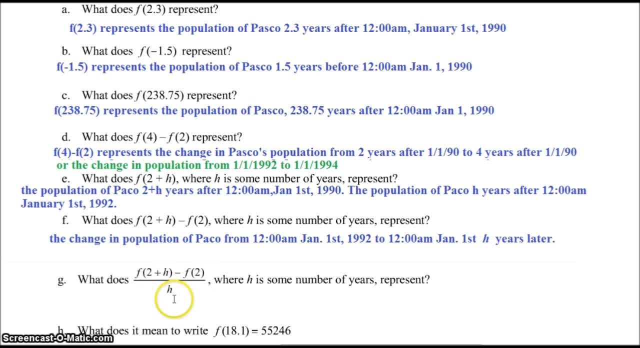 So what does f of 2 plus h minus, f of 2 over h, where h is some number of years, represent? Notice that this function would give us a change in population divided by a change in time. So this is a rate. 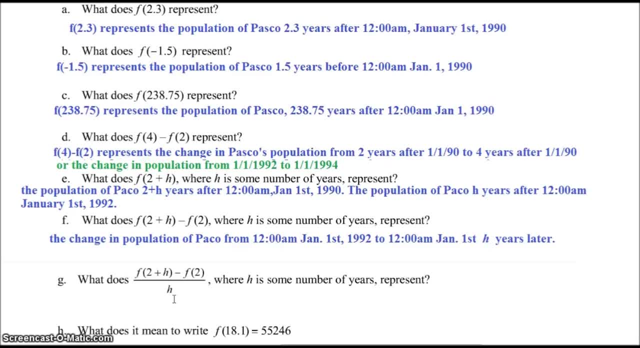 It's a ratio, It's a. it's a rate of change. Okay, More specifically, it's the average rate of change of the population of Paco Washington from 2 years after January 1, 1990 to 2 plus h years after January 1, 1990.. 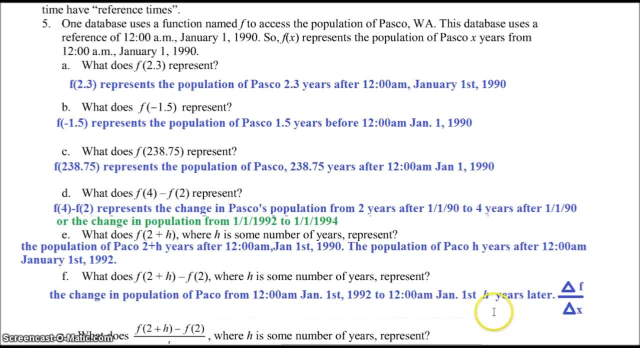 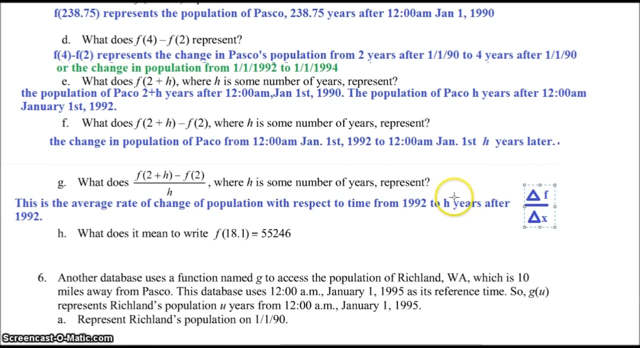 Okay, Okay, Okay, Okay. So, oops, I put that in the wrong spot. Grab this. So f of 2 plus h minus f of 2 over h. I said that's the average rate of change of population with respect to time from 1992. 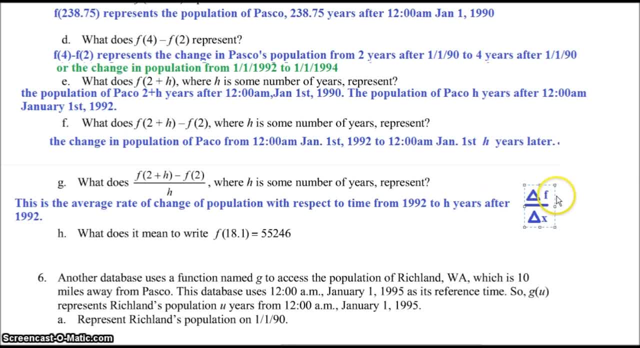 to 8 years after 1992.. It's simply a change in the function values or a change in population over a change in the input values, a change in time, delta f over delta x. And remember the average rate of change is the constant rate of change we would need. 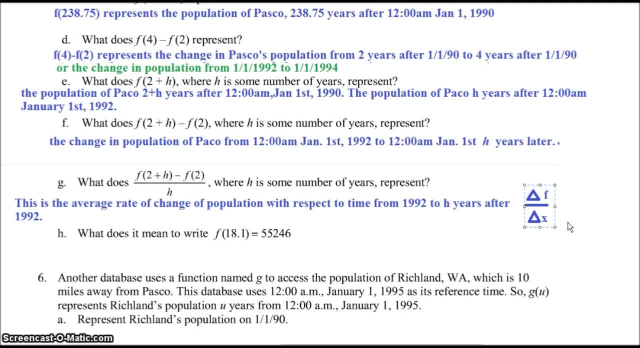 to have the same increase in population or same change in population over that time interval, h. So what does it mean to write: f of 18.1 equals 55,246? That simply means that 18.1 years, 18.1 years after January 1, 1990, the population of Paco was 55,246. Number 6.. Another database uses a function named g to access the population of Rayleigh, Number 6.. The population of Richland, Washington, which is 10 miles away from Pasco. The database uses 12 am January 1, 1995 as its reference time. 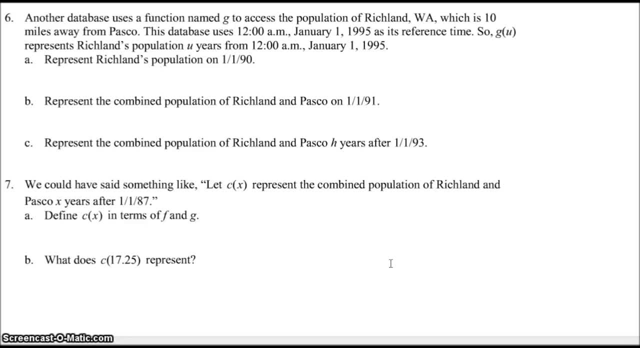 So g of u represents Richland's population u years from 12 am January 1, 1995.. Represent Richland's population on 1,190.. So notice that 1,190.. Well, that was the. 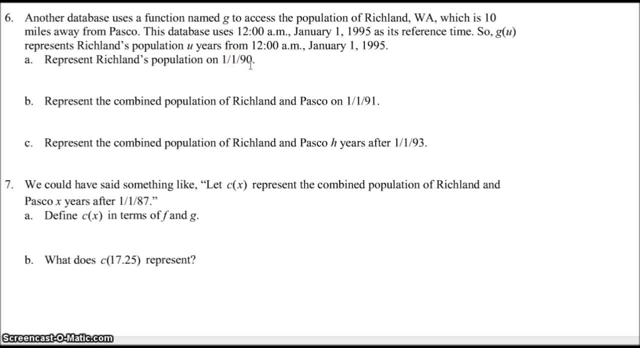 starting time or the reference time for our previous problem in number five. now our reference time is January 1st 1995, so that's like our zero position. so we actually are going five years in the past. so that'll be a negative five for our. 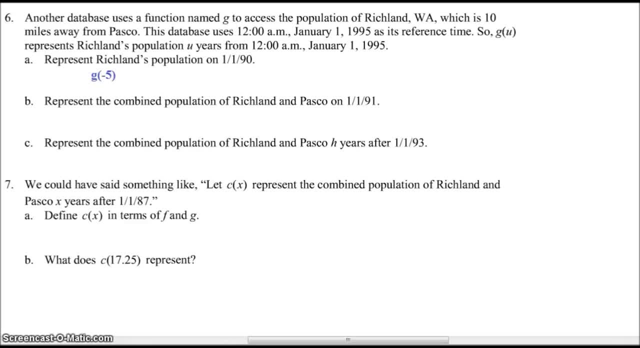 input and we can express that as G of negative five. so G of negative five represents his population five years before January 1st 1995, which will be on January 1st 1990. represent the combined population of Richland and Pasco on the 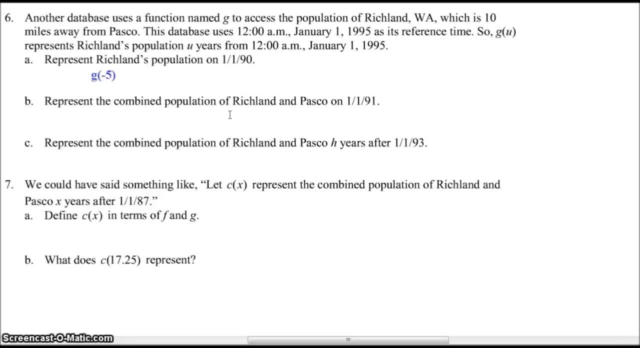 1st of January 1991. so for Pasco- that's from the previous question- that'll be F of one, because we're one year after 1990, and for Richland in 1991, that's four years before our reference point. so that will be G of negative four. now 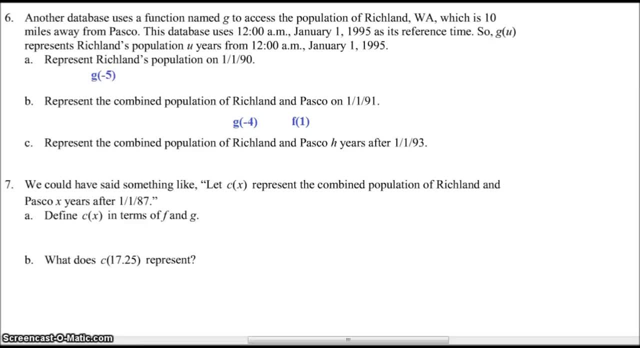 we want the combined population of Richland and Pasco on that date. so we simply take the population of Richland and add it to the population of Pasco. G of negative four plus F of one, that's the combined population of Richland and Pasco. 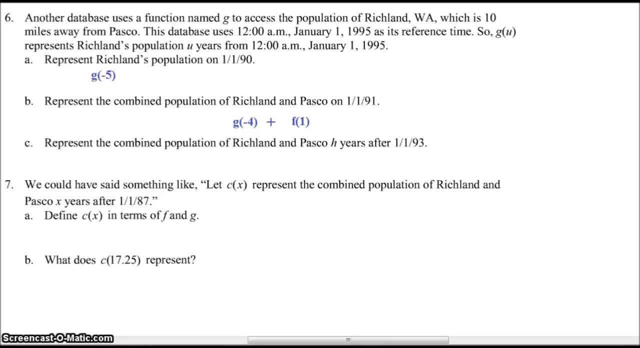 on January 1st 1991. part C represent the combined population of Richland and Pasco eight years after the 1st of January 1993. so with Pasco eight years after 1993, well, 1993 is already, let's see, three years after our reference point. 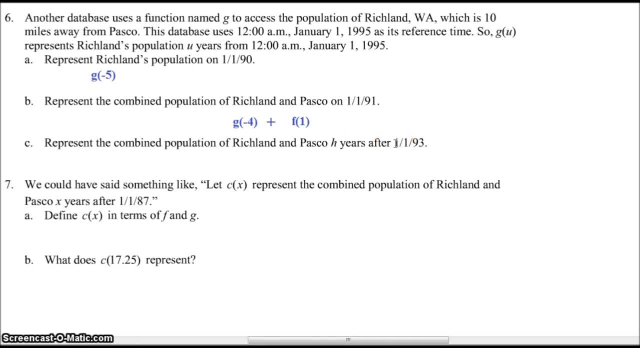 so we can represent the population eight years after 1993 as F of H plus three for Pasco and for Richland, that's two years. 1993 is two years before our reference point of 1995. so we're basically going a negative two year. 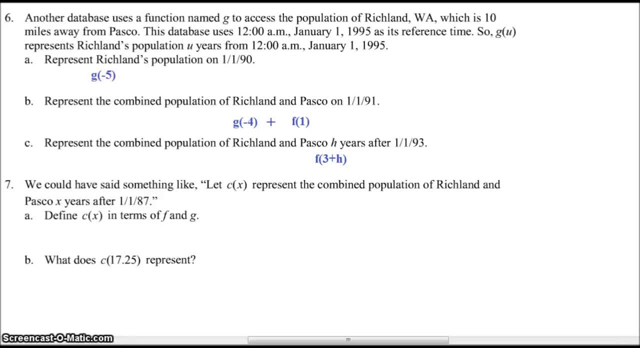 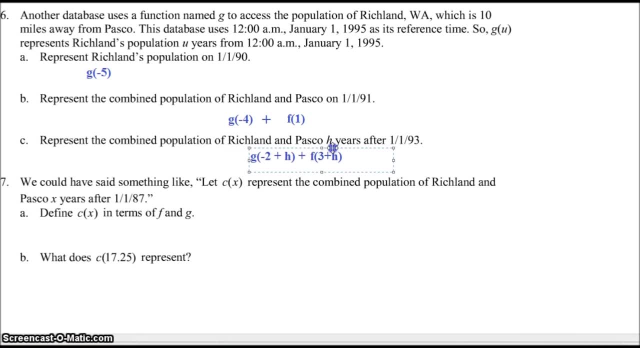 to that. that will simply be G of negative 2 plus H, and since we want the combined total, we simply add these G of negative 2 plus H plus F of 3 plus H. again, the G of negative 2 plus H is Richland's population two years before. 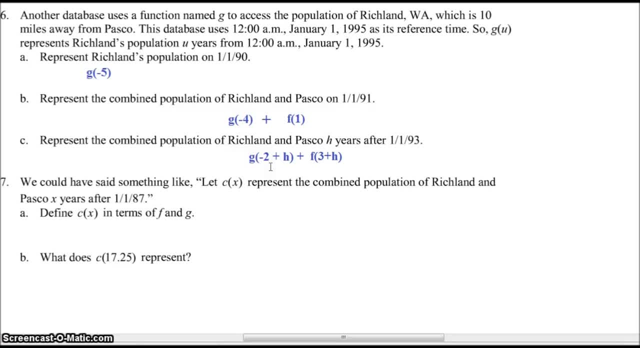 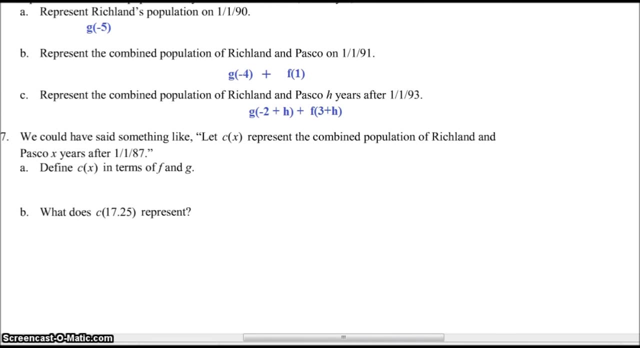 before 1995 and then eight years after that. and here we have Pasco: the population three years after 1990 plus eight years after that. number seven says we could have said something like: let C of X represent the combined population of Richland and Pasco X years after 1187. part a says: 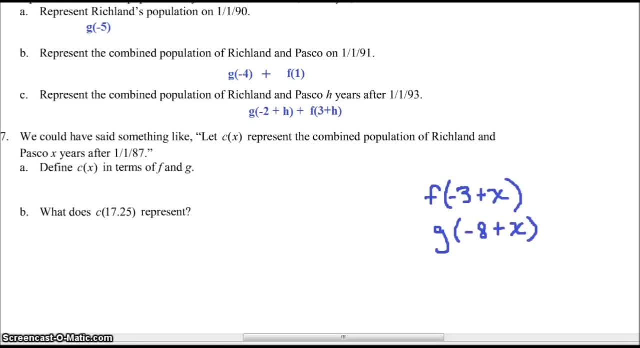 define C of X in terms of F and G. okay, this problem you'll have to think about for a minute. so I went off and did some side work over here. if I want 1987 to be my new reference point, then that's going to alter my functions a bit because I need- well, let's see what- 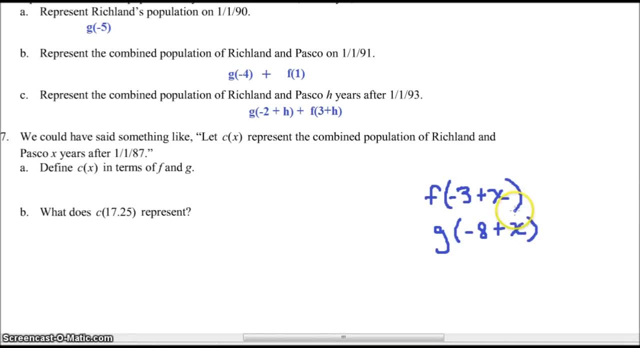 we need. take a look at F. this is for Paco. if I plug 0 in for X, that will give me the value of Pasco's population in 1987. F of negative 3, and then if I skip up to X, equals 3. 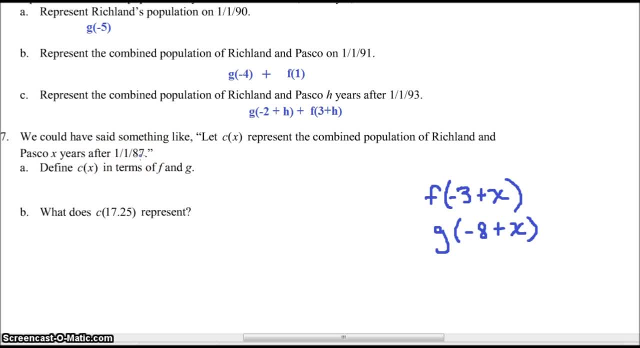 that'll be three years after 1997, that will be 1990, and then I'll get back to normal. I have F of 0. same thing here with G. 1987 is eight years before 1995, the reference point for G, so we can. 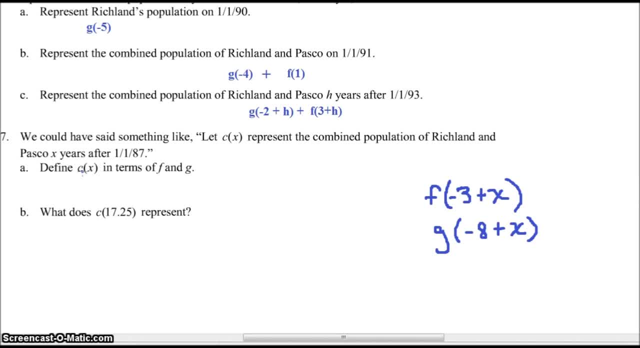 combine these two functions to get C of X, you and H and G. we work with like 1990 and Royce, you know the range of values of a numerical story, but what I was trying to show here is this was something that you can do, influenced, or you might be able to estimate an. 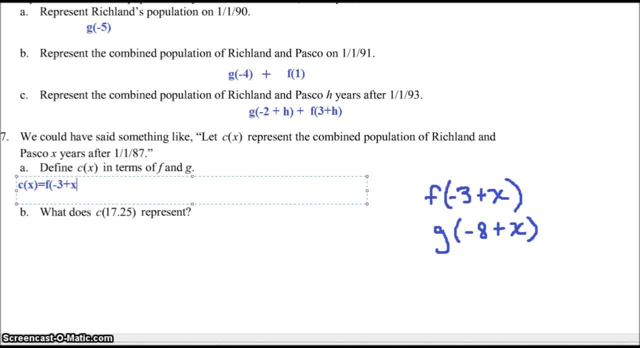 interpretation of what somebody is going through, what it looks like and I have been doing it or anything I talk to them. he might fall into this in John Jackson racism or some Psych BehavioristÓ, whatever you guys want, but I think that makes you kind of feel like you're. 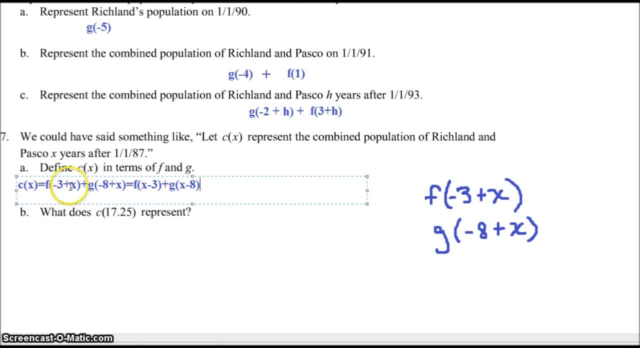 kind of stuck in thebedingt revolution of rock profit. so I'm kind of esperando more questions and answers, if a's anything like that, and then you'd remember us Okay. so either one of these expressions will work: f of negative, 3 plus x plus g of negative. 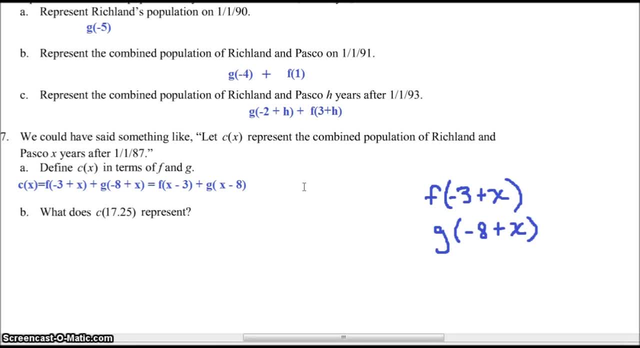 8 plus x. that's equivalent to f of x minus 3 plus g of x minus 8.. This is a tough problem. You might need to have some more time to think about this one. What does c of 17.25 represent? 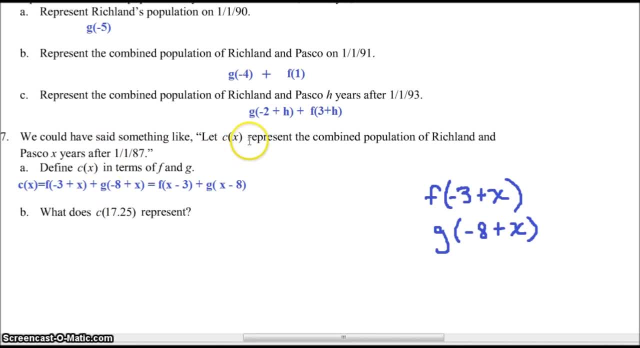 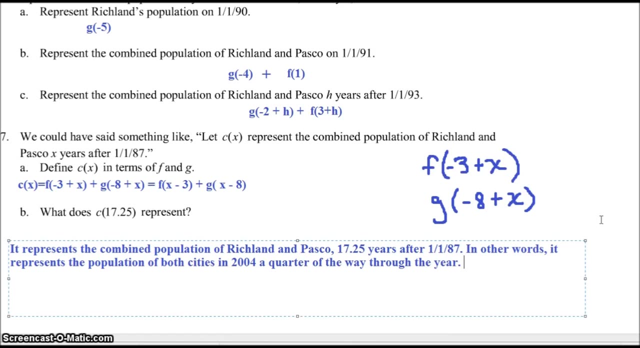 Well, that, just based on our definition here, represents the combined population of Richland and Pasco x years, or 17.25 years after 1987.. Okay, So it represents the combined population of Richland and Pasco 17.25 years after January. 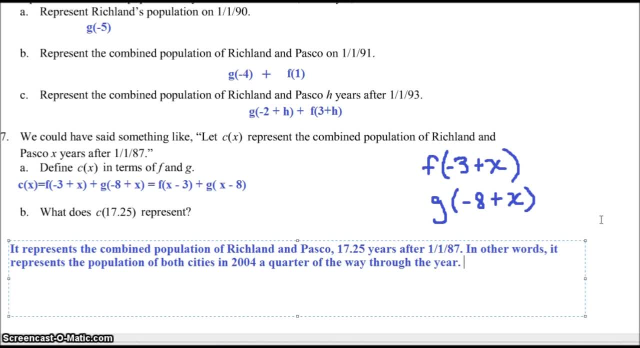 1, 1987.. Now if we add 17.25 years onto 1987, we get to 2004,, and that .25 tells us we're a quarter of the way through the year. Now we need to represent the combined population. 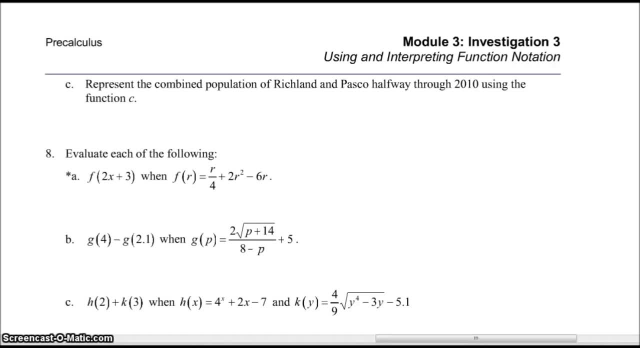 We need to represent the combined population of Richland and Pasco halfway through 2010 using the function c. So halfway through 2010 tells me we're going to need a .5 on our answer, And then we just need to subtract 2010 minus 1987.. 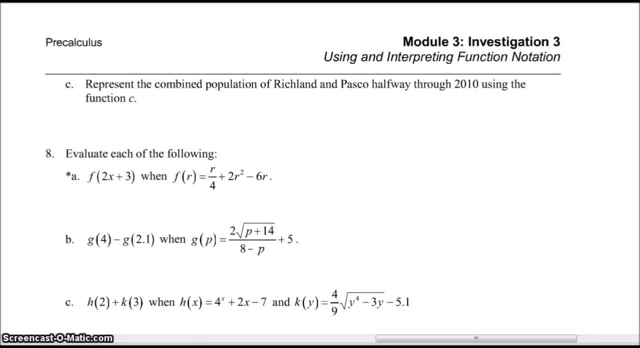 So you can check: 2010 minus 1987 is 23.. So we're 23 and a half years after 1997.. That's c of 23.5.. And that's how we represent the combined population. Okay, So that's the combination of Richland and Pasco halfway through 2010. using the function. 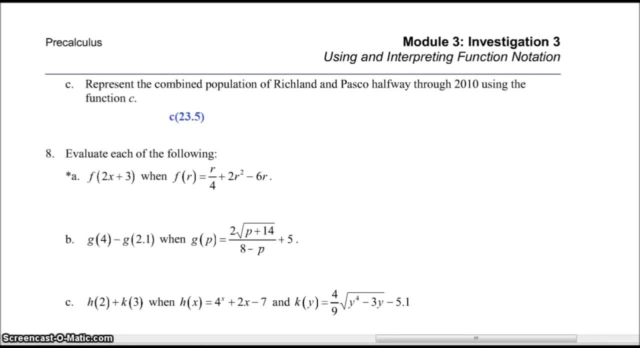 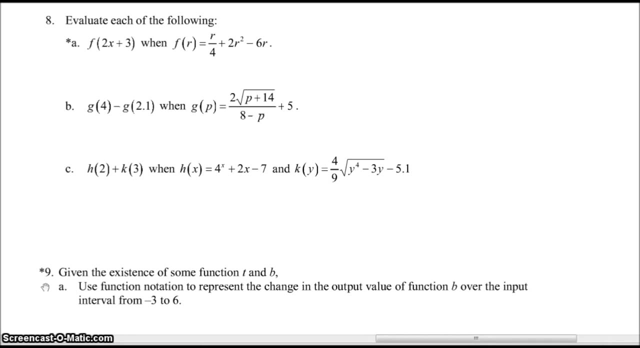 c And we could plug in that number to the function c and get a value if we wished. Number eight: Evaluate each of the following: Part a: F of 2x plus 3.. When f of r equals r over 4.. 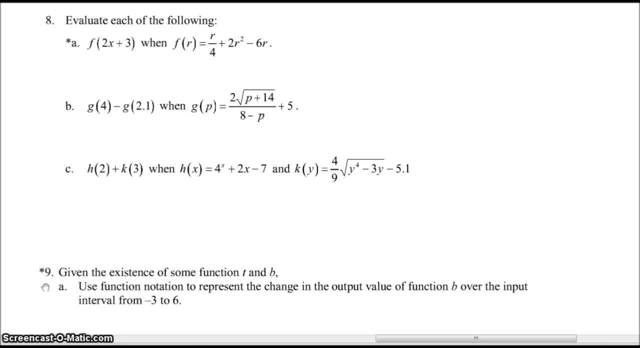 Plus 2r squared minus 6r. So don't be afraid of this one. Just take a second and think about what it's asking us to do. We have a function f in terms of an input r, And you can see that the value of the output is determined by this rule. 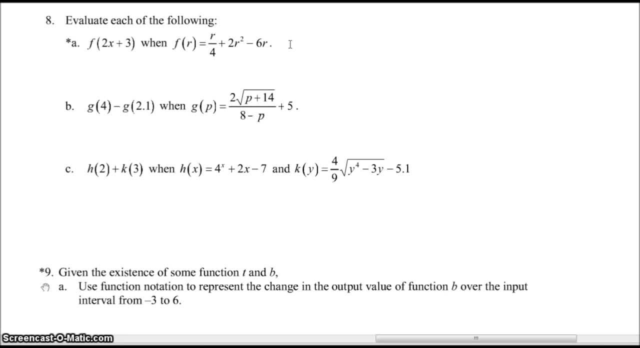 r over 4 plus 2r, squared minus 6r, And we would just want to find the value of the output, f, when the input is 2x plus 3.. So we simply replace r with 2x plus 3 everywhere here in the expression. 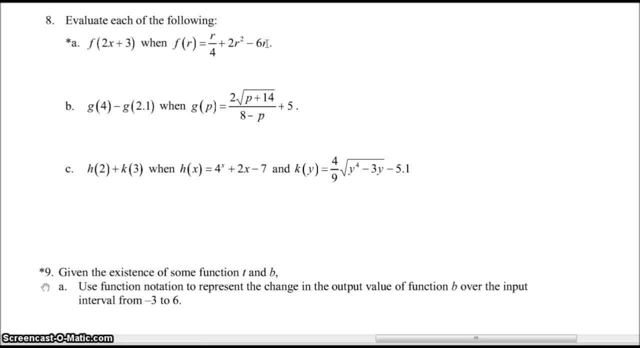 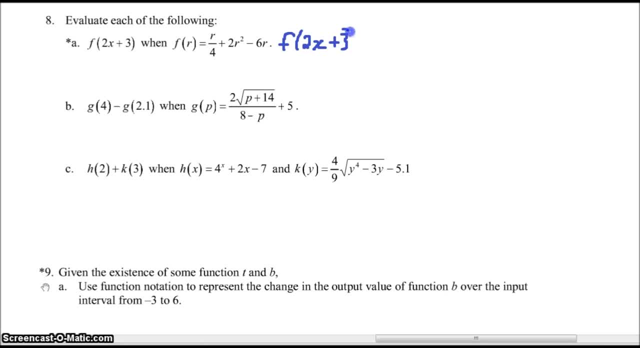 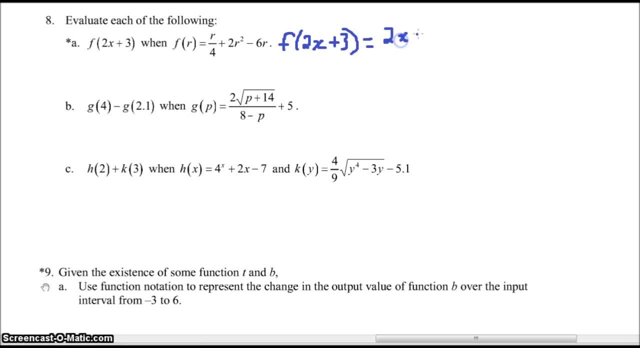 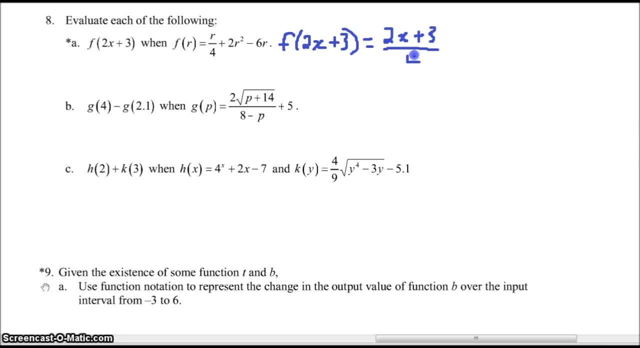 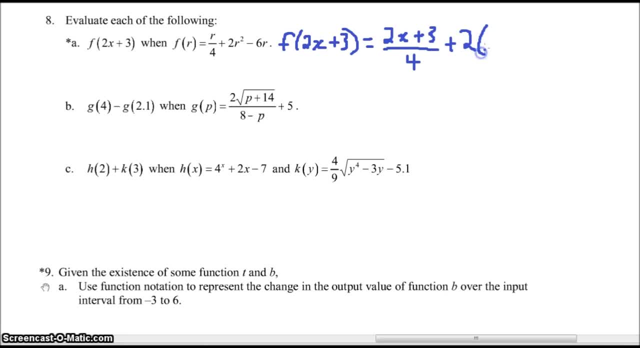 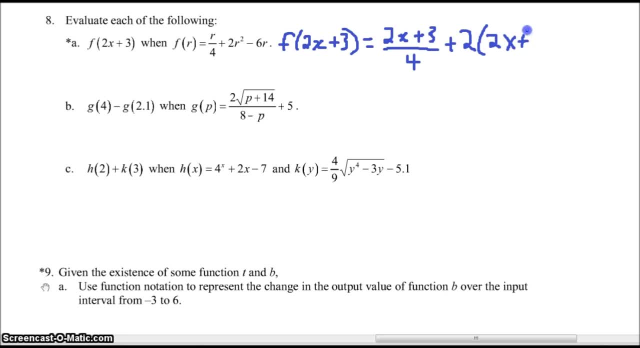 F of 2x plus 3.. And then minus 6r, But instead of r we're going to write 2x plus 3.. We've substituted 2x plus 3 into our function. The next problem asks us to find g of 4 minus g of 2.1, when g of p is 2 square root of p. 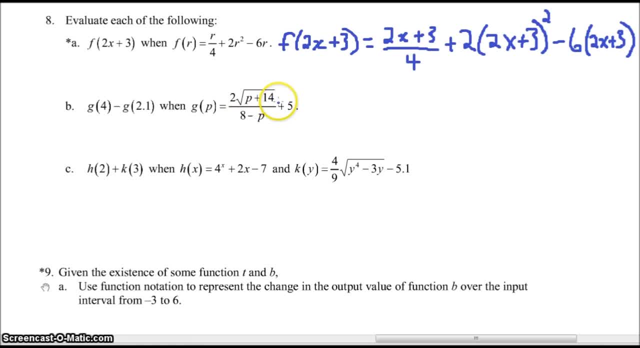 plus 14, divided by 8 minus p plus 5.. So all we've got to do is substitute 4 into our function, make 4 the input, Find the result and subtract 2.1, not 2.1, subtract what we get when we plug 2.1 into. 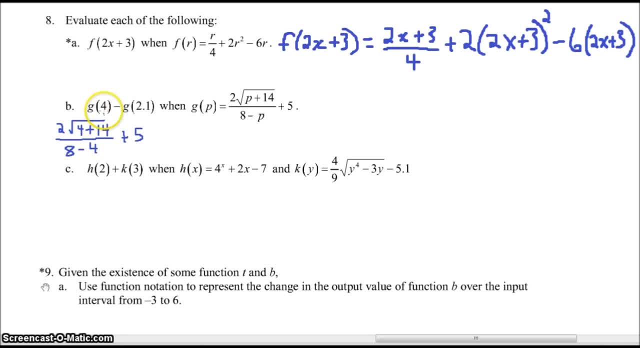 our function. So note here that I've just calculated g of 4.. I've plugged in 4 in for p. 4 is my input, 2 square root of 4 plus 14 over 8 minus 4 plus 5.. 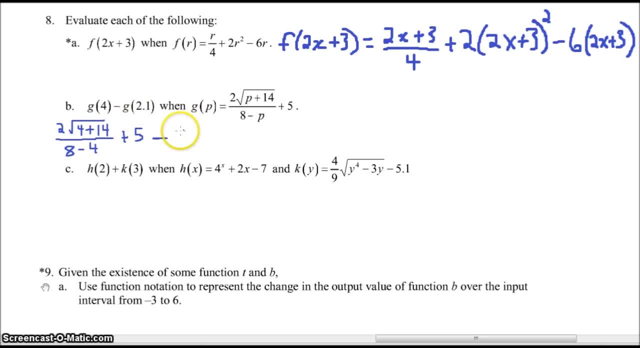 Now I need to subtract g of 2.1, which is just 2 square root of 2.1.. Plus 14, all over 8 minus 2.1 plus 5.. Now it's really important here that I put parentheses around this whole expression, because 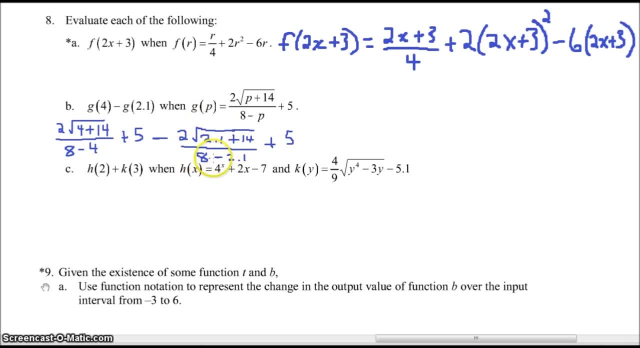 notice if I don't. I'm just subtracting this first part of our expression, but I'm really subtracting g of 2.1, which is this whole piece. It's crucial that you put the parentheses there. If you don't, you'll get the answer wrong. 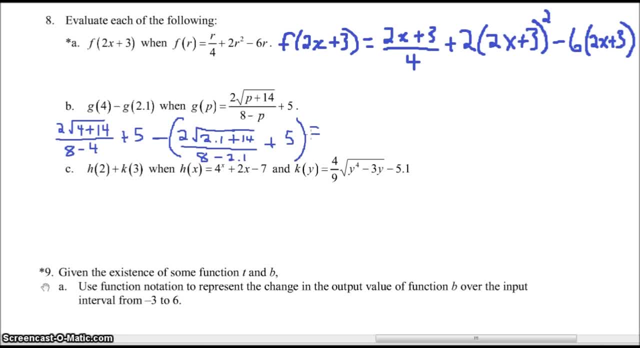 Now just use your calculator and figure out what the value of this expression is. It should get something like .7612 approximately. All right, Let's try part c, H of 2 plus k of 3.. 4 raised to the x plus 2x minus 7 and k of y is 4 over 9. square root of y to the fourth minus 3y. 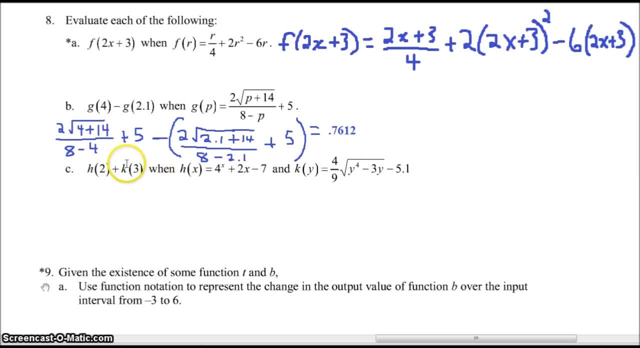 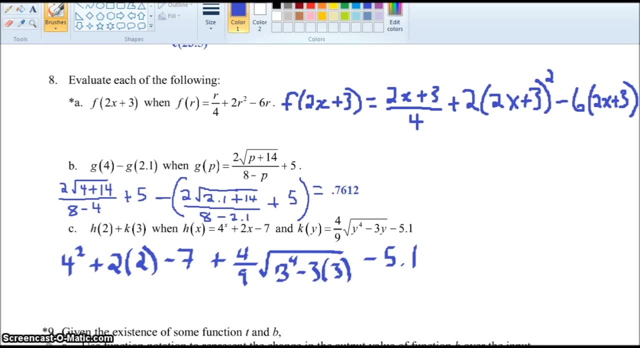 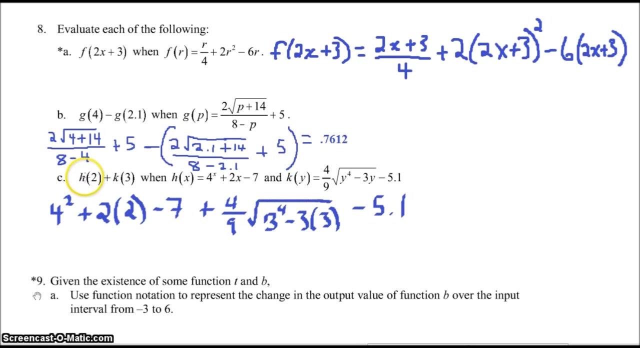 minus 5.1.. All we're doing is taking 2 and substituting it in for our input x and taking 3 and substituting it in for our input y, as follows: All right, so notice that I've simply taken h of 2, which is h of x, but with a 2 in place of the x. it's 4 squared plus 2 times 2. 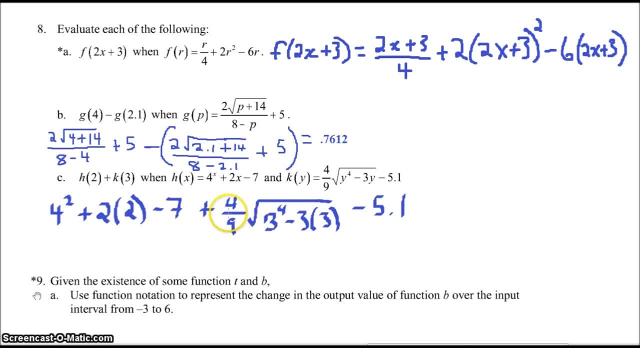 minus 7.. And then k of y is k of 3, that's 4 ninths square root of 3 times 2 minus 7.. And then k of y is k of 3, that's 4 ninths square root of 3.. 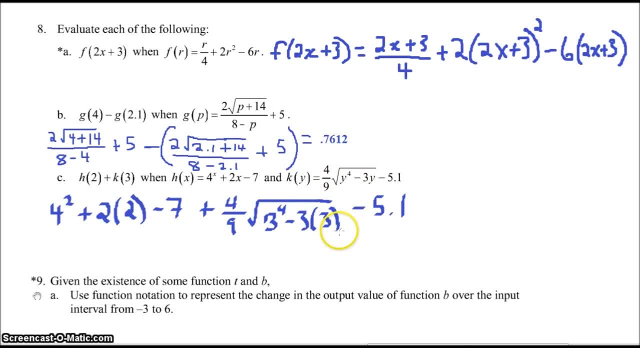 to the 4th minus 3 times 3.. I just replaced these y's with a 3 and subtract 5.1.. And then that should come out. just use your calculator. I think this comes out to 11.67.. 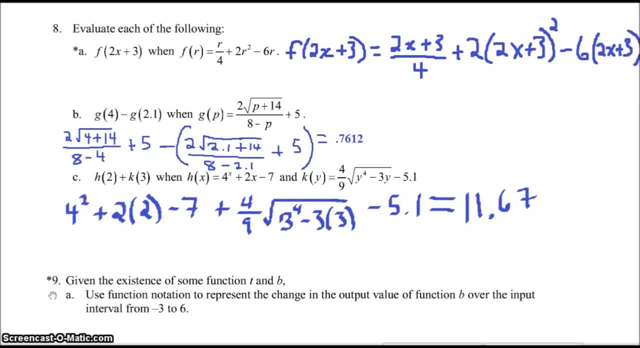 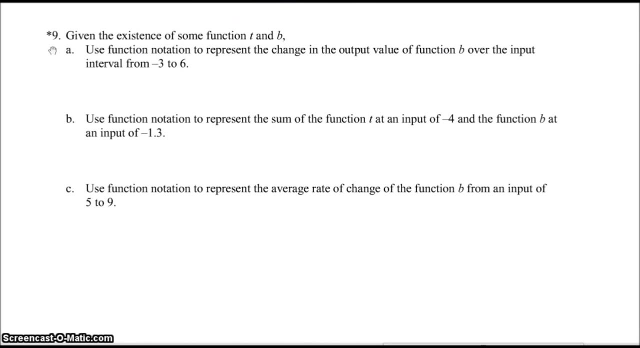 The book's answer is 14.5,, but I can't get that. I don't know how they got that one, So check this yourself. Make sure you can get a good answer for this one, Number 9,, given the existence of some function: t and b. 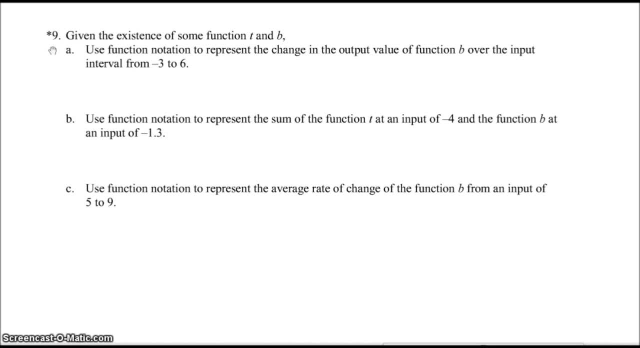 I'm guessing that means there's two functions. use function notation to represent the change in the output value of function b over the input interval from negative 3 to 6.. So remember that a change in the output value of function b is a change in the output value. 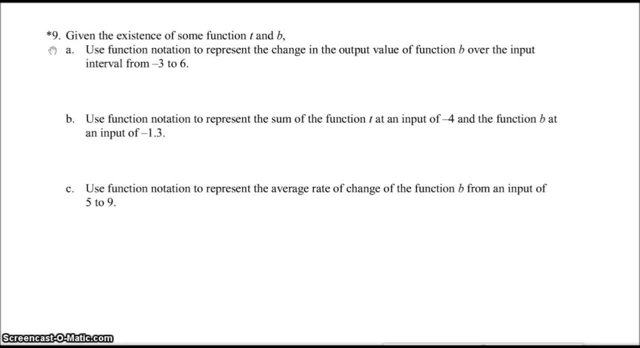 of function b over the input interval from negative 3 to 6.. So remember that a change in the output value is just the final value minus the initial value. So here the input's changing from negative 3 to 6, so we simply need b of 6 minus b of negative 3..